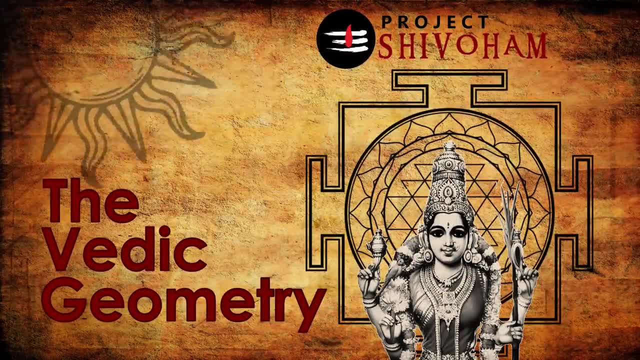 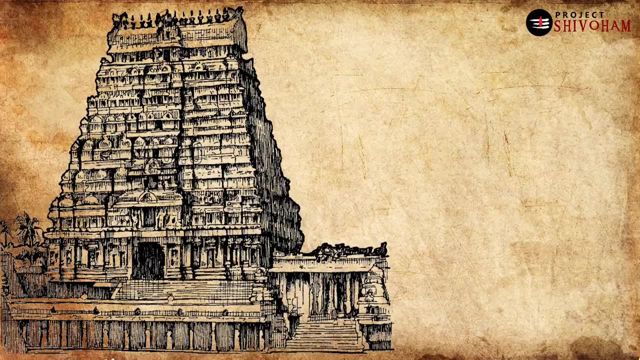 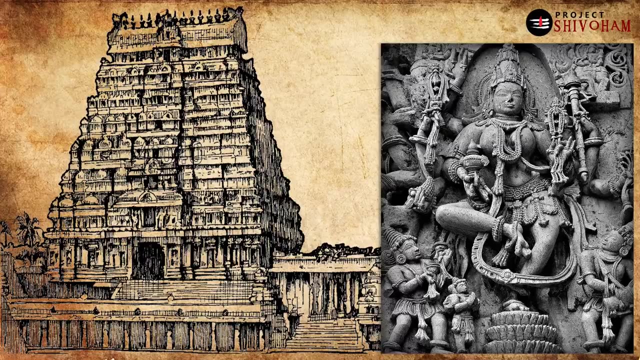 Temples are the heart and soul of Indian culture and heritage and they stood the test of time since thousands of years. The grandeur of the sculptures on these temples, its architecture, the way they are built- thousands of years ago just unparalleled. Well, it's very difficult to just draw a perfect. 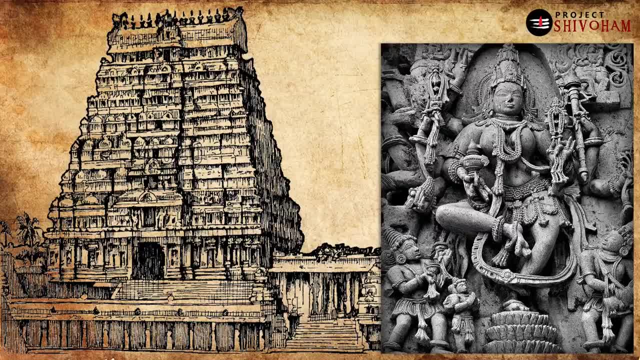 circle with a free hand, What could have been the geometrical expertise of people back then who built these grand structures? That was the question we had, and this video is a result of our attempt to understand what has been the Vedic geometrical expertise of ancient Indians To set. 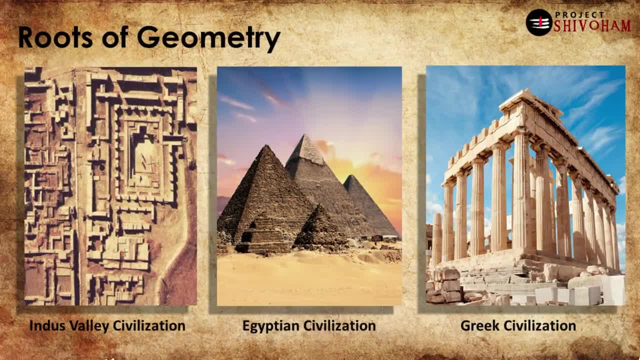 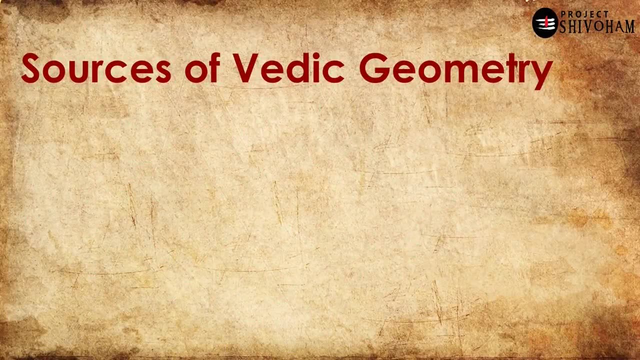 the context, geometry is a very natural thing. Almost all the civilizations express their culture and heritage in some form or shape in which geometry takes the center stage. This video is purely to understand from an ancient Indian standpoint what was their expertise with respect to geometry back then, For ease of expression, we picked up the word Vedic geometry as broadly to 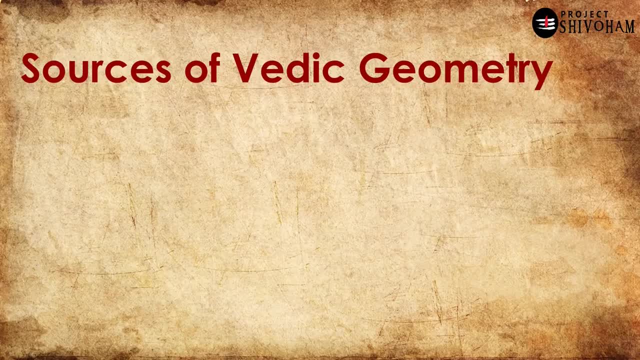 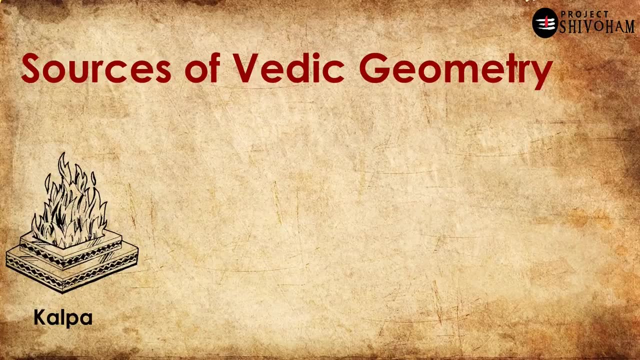 encompass geometry as described in all the ancient Indian scriptures. So the first place where we find the Vedic geometry applications is in Kalpa. It deals with executing the Vedic rituals of Yajnam for different purposes. The second place where we find geometry 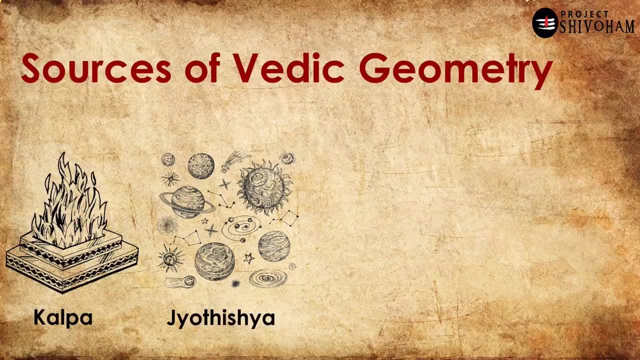 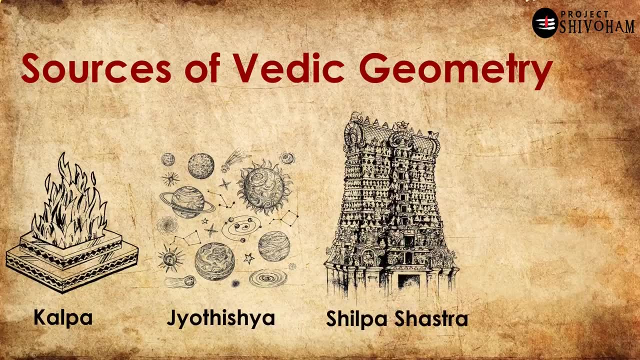 is in Jyotisha. It deals with astronomical studies that's essential for a Vedic culture. Moving next, in the third place, where we find geometry is in Shilpa Sastra, a branch of knowledge that deals with the temple construction and sculpting. The fourth and the last area where 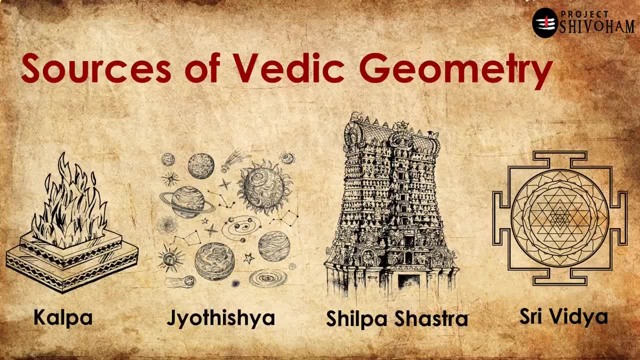 we find geometry is in Srividya. It is a specialized branch of divine worship which is broadly categorized as Tantra, but for ease of expression we'll use the word Srividya. It deals with construction of complex two-dimensional and symmetrical geometrical diagrams that are the 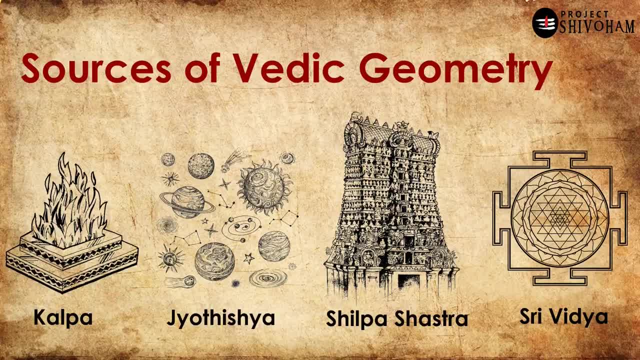 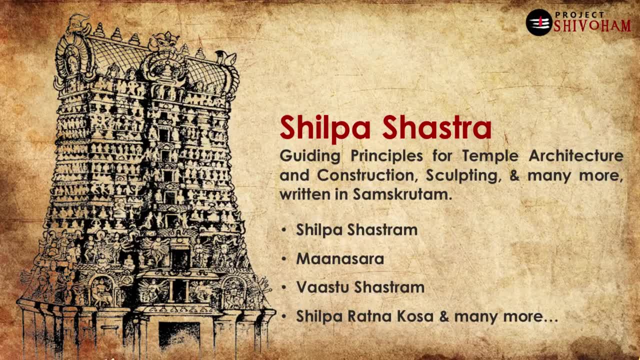 manifestations of different gods, And this documentary is about how geometry thrived in these four areas since times immemorial. Let's briefly flip over these four, starting with Shilpa Sastra. Shilpa Sastra is a very broad term which is generally used for categorizing all the 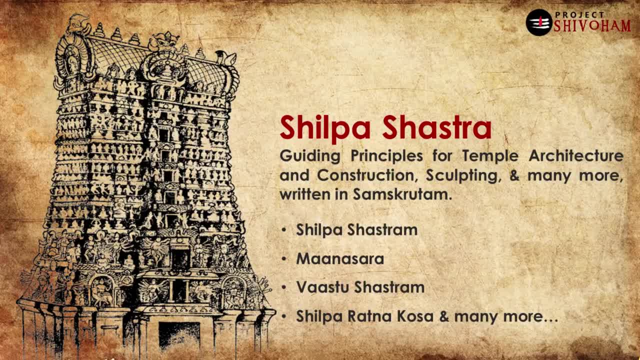 scriptures that deal with the temple: construction, sculpting, metallurgy, architecture and a lot more. There are many scriptures under Shilpa Sastra, like Manasara, Vastu Sastram, Shilparatnakosa and many more- All the geometrical principles that are needed for. 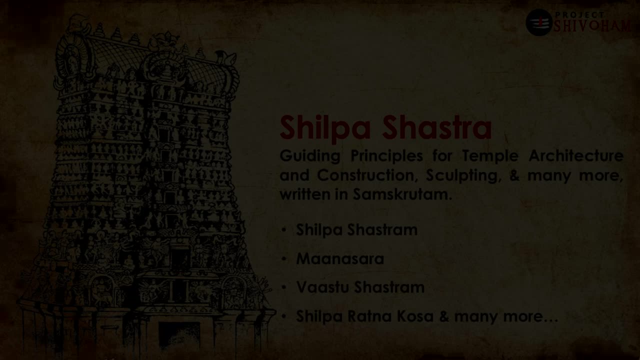 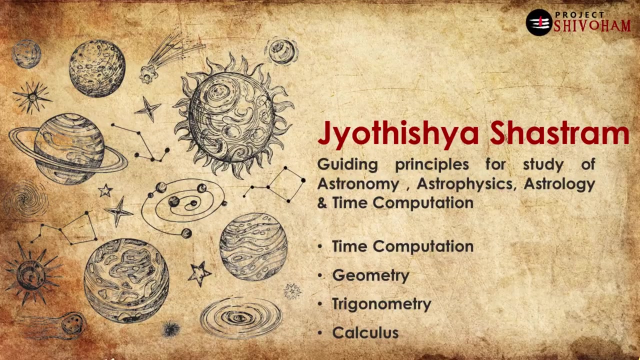 temple construction are explained in these scriptures. Up next is Jyotisha. This is one of the most misunderstood branches of knowledge, that it's about future prediction, etc. etc. But Jyotisha, the word literally means study of light. It deals with computation of planetary positions. 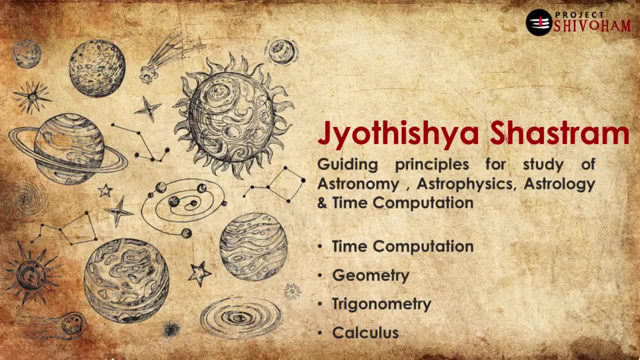 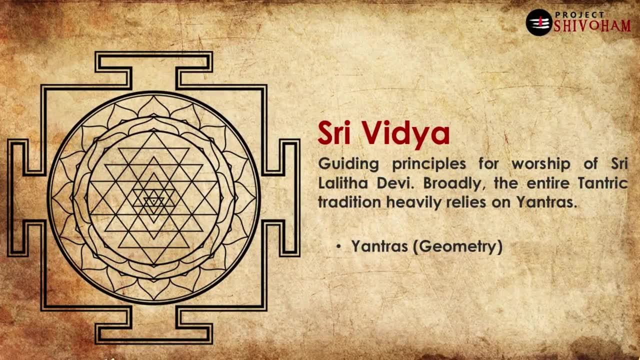 and as part of it, there are a lot of geometrical principles that are detailed out in the scriptures. We'll see them as well in this video. In India, when it comes to divine manifestation, gods are always depicted in forms of sculptures. 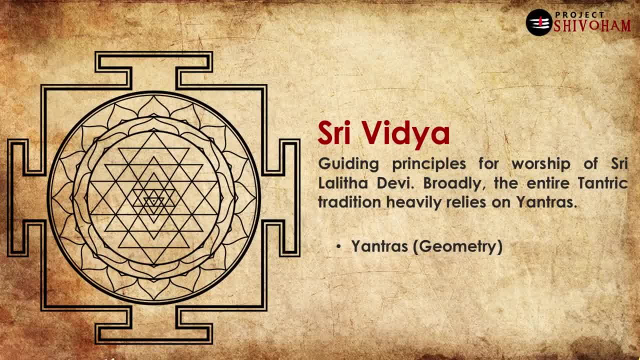 or murtis, And that's what we generally see in the temples. But there is another practice where the divine incarnations of gods are manifested in the form of a two-dimensional symmetrical diagrams. So Srividya details about construction of these complex geometrical figures. 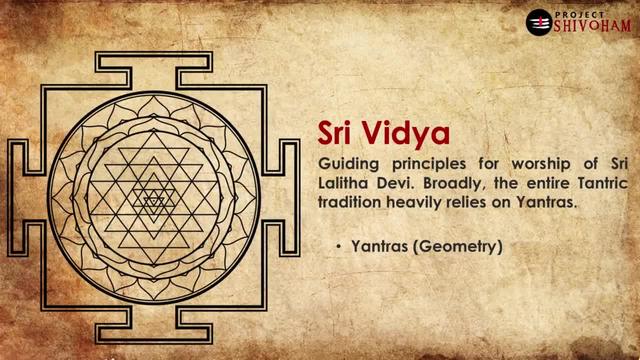 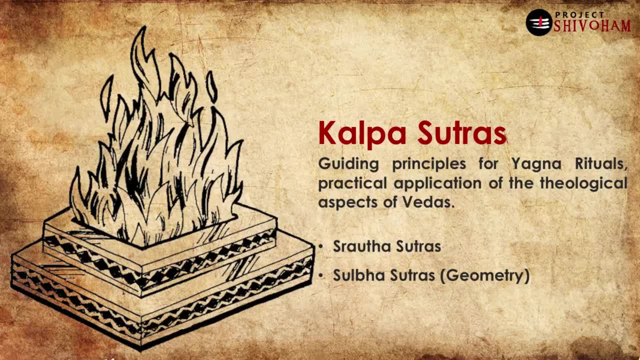 which deals with different geometrical shapes and the principles behind them. The fourth one is Kalpa. Kalpa deals with setting the guidelines for execution of the Vedic rituals like Yajnaam, And you might have seen the fire altar, which is typically in a square shape, like 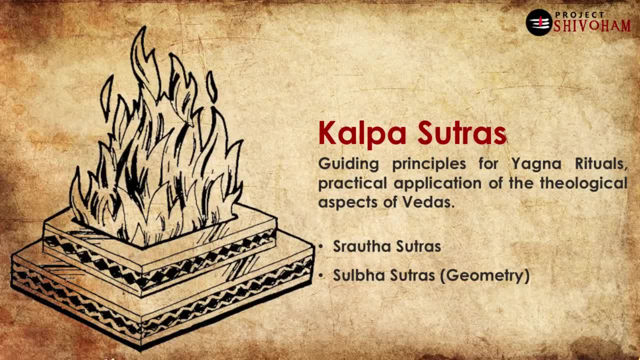 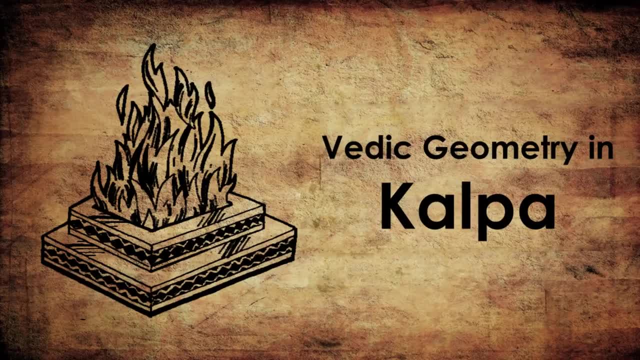 third one is the Kalpa, The fourth one is the Kalpa, The fifth one is the Kalpa And the third one is the Kalpa. So let's start with the first one, Kalpa, How the Vedic geometry is defined in Kalpa. 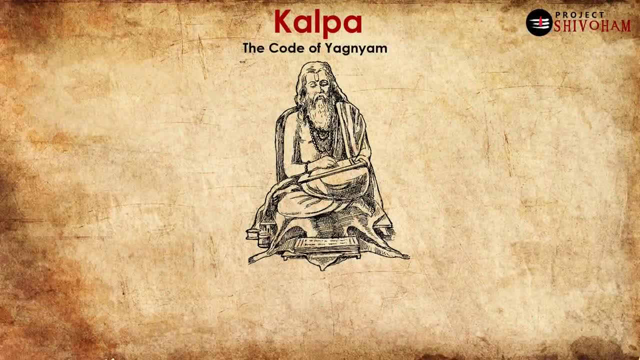 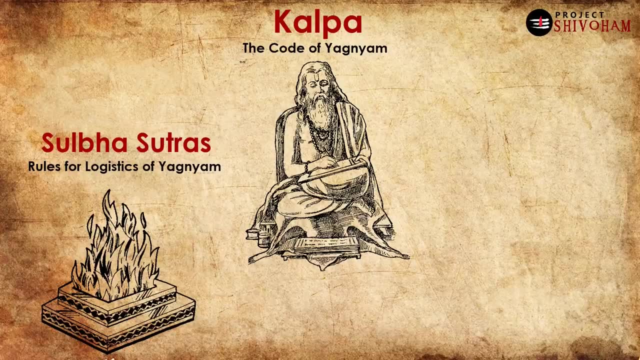 So Kalpa is the code of Yajnaam. It has all the rules and regulations and bylaws related to how you execute a Vedic ritual, And it has two parts to it. The first one is Sulbha Sutras. This: 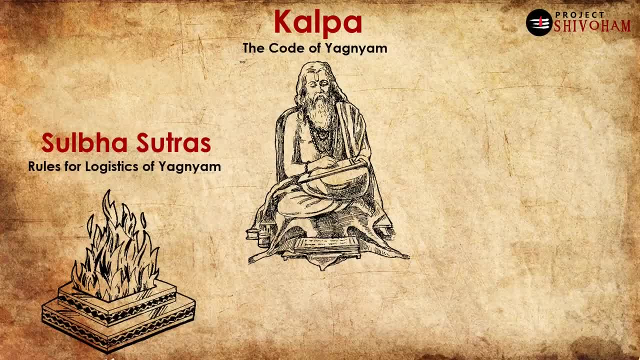 talks about the rules, of the logistics that are needed for Yajnaam, as to how you construct these fire altars, the Yajnaashalas, and a lot more. And the second one is Shravata Sutras, which contain: 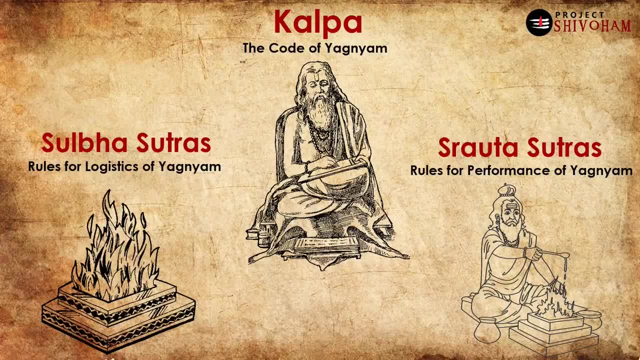 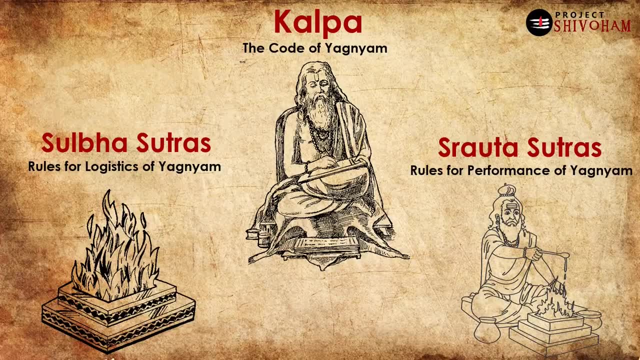 the mantras and the Vedic hymns which are needed for the execution of Yajnas, the ritual. So Sulbha Sutra is about preparation and Shravata Sutra is about execution, and you'll get to know in a minute why we are talking about these. 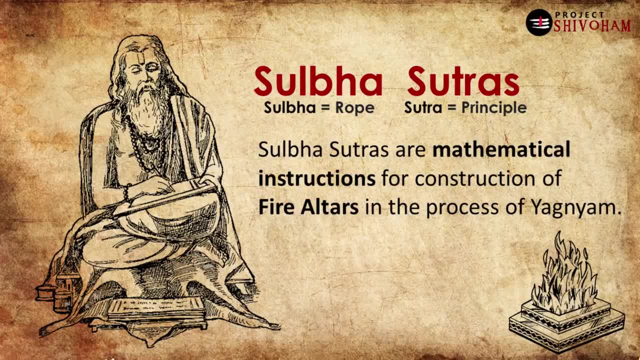 Sulbha Sutras. it's two words: Sulbha and Sutras. Sulbha means rope and Sutras means principles. So basically, these are the mathematical instructions that are crucial in construction of the fire altars in the process of yajna. 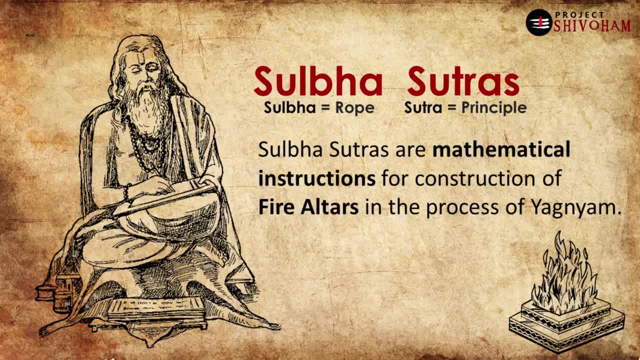 Thousands of years ago they did not have scales like what we have now, So a rope is used as an instrument to measure any surface, and hence with that name goes Sulbha Sutras. In simple words, these are the geometrical principles. 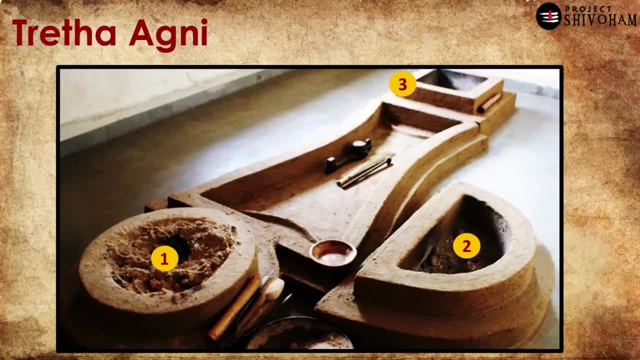 The concept of Yajnam is a very, very ancient practice which has been thriving in India. since no one knows, when You take any kind of ancient Indian scripture, you will not find it without reference to some kind of a Yajnam, such as the antiquity of this ritual. So what you're seeing on the screen is a relic of one. 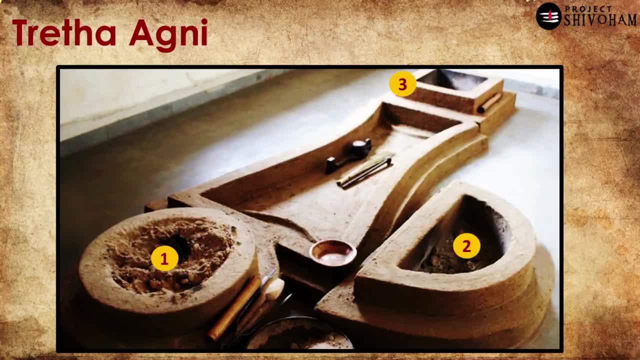 of such. As part of one of these rituals, there are three fire altars that should be maintained in every household. back then It is called as Treta Agni, or, in simple words, three fire altars. They are Ahavaniya, Grahapatiya and Dakshinagni, as you're. 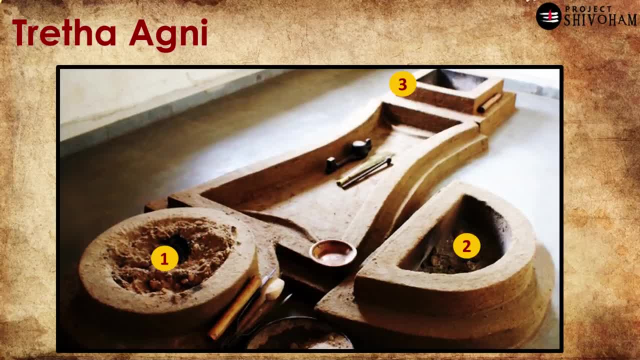 seeing in the markings, As you see the shapes: they are circle, square and semicircle. The most important aspect here is there is a very strong constraint which says that all these three fire altars should have exactly the same area. Now I don't know what is the religious significance behind that. 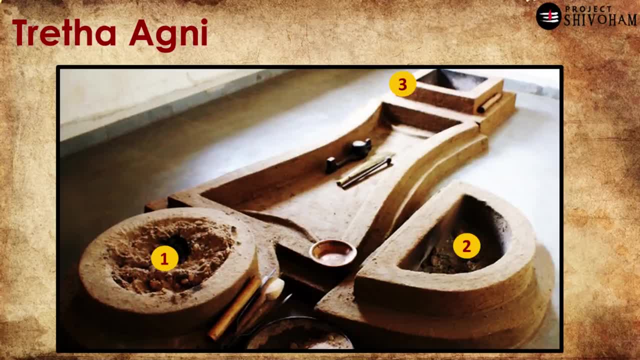 constraint, but all these three, if constructed at a place, should be exactly of the same area. This might not sound as a big deal to you now, because we have all the formulas invented for calculating the areas of these shapes, but thousands of years ago geometry was totally in a different format. So how? 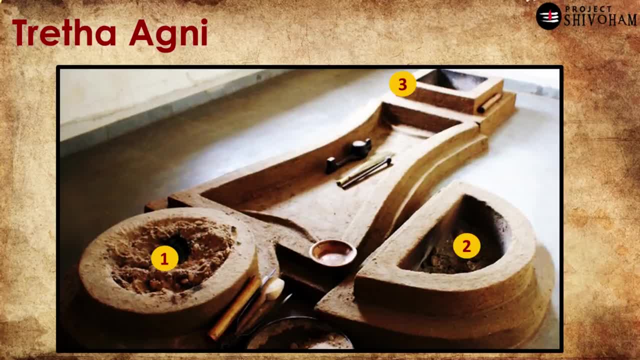 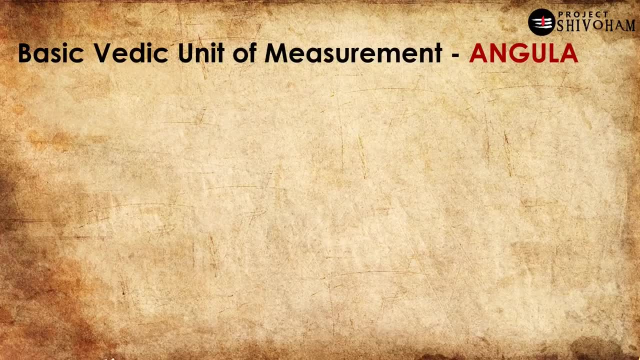 did the ancient Indian rishis manage to measure areas of these kind of fire altars thousands of years ago? Now let's see Talking of measurement. the first thing is unit of measurement. So what was the unit of measurement? unit of measurement back then? it is angula. this is the basic unit of measurement, as per sulbha sutras. 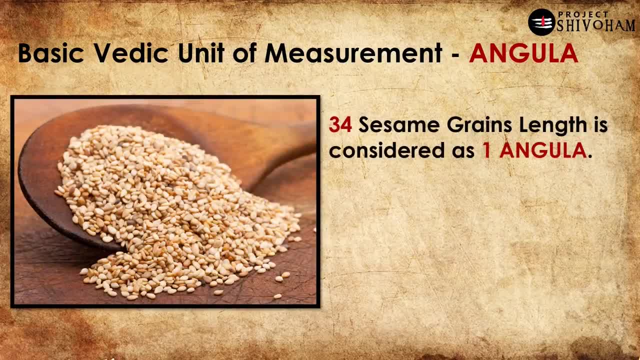 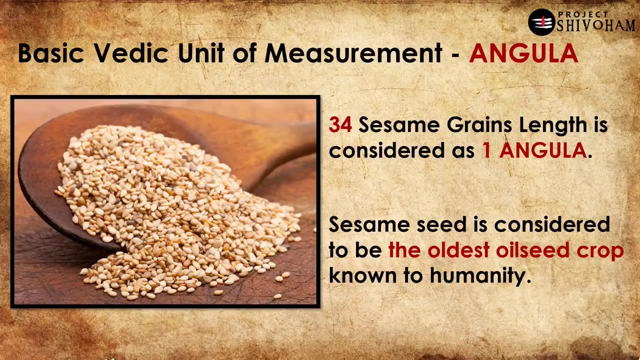 34 sesame seeds stacked up against each other in a line that is the length of one angula. that was basically the unit of measure of people back then, so that comes around four to five inches, as per our inches today. also, sesame seeds are one of the oldest known sources of oil to humanity, so 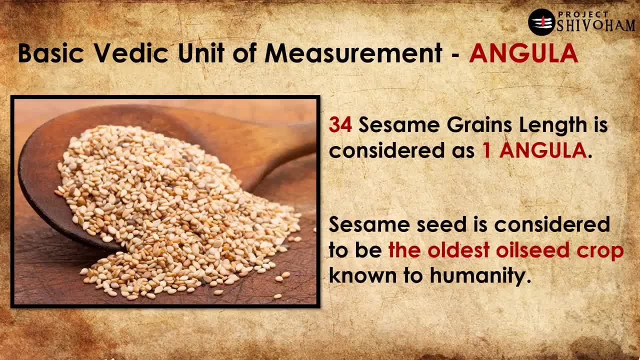 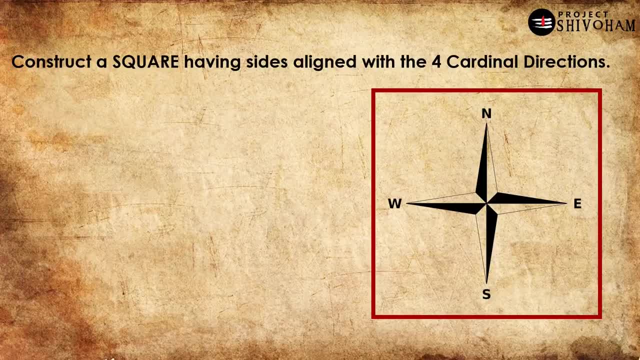 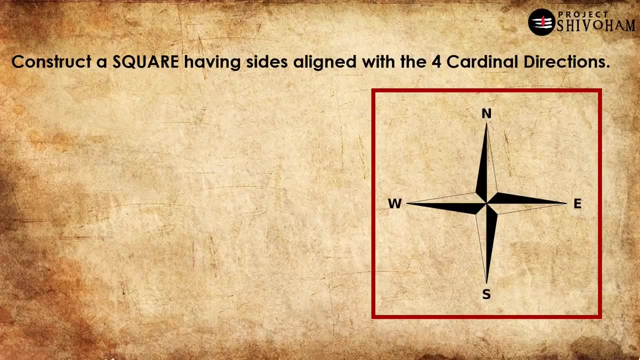 that also explains the antiquity of the vedic rituals and the time they belong to. let's take a very simple problem: to understand how the ancient indian people constructed these fire altars, can you draw a square with its sides perfectly aligned with the four cardinal directions? you would need definitely a pencil, compass paper and a scale. without these we cannot. 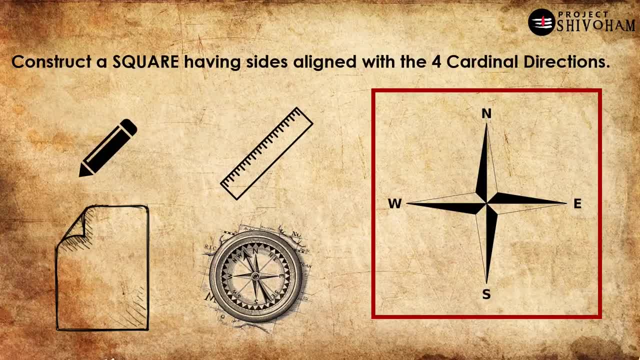 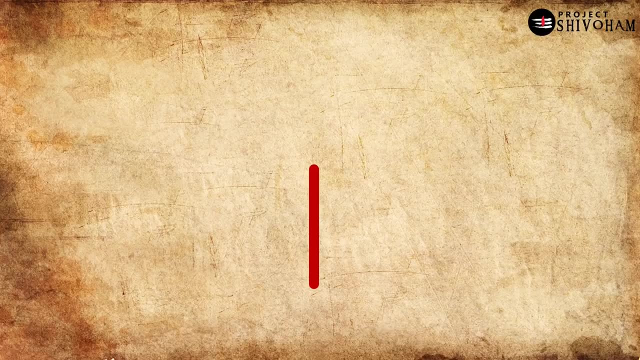 draw a square with its sides perfectly aligned with the four cardinal directions. it's a simple thing, right? but back then none of these were available: no compass, pencil or scales. so how did they go about it? let us see. so, first things first, identifying the four cardinal directions. these are not fixed. because of the solstice. the sun movement varies from. 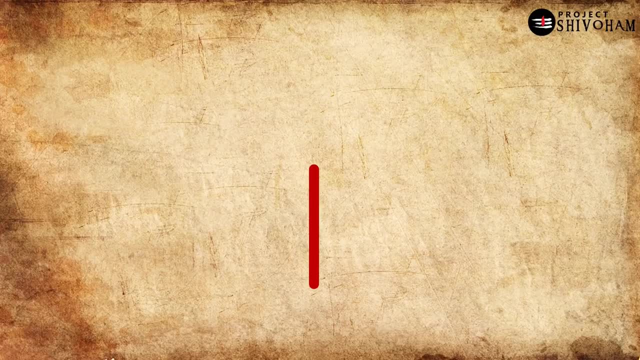 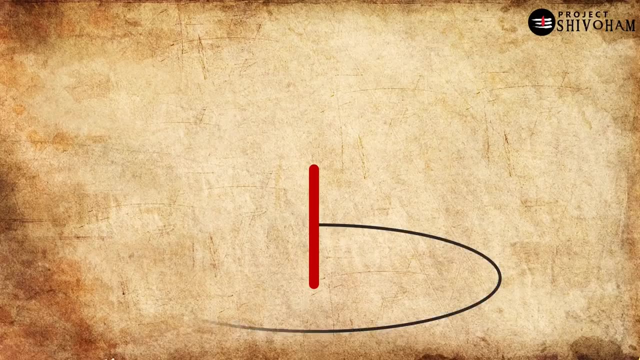 season to season right, so we need to get the directions which are applicable on that day of the execution of this ritual. so here is how they did: they took a long stick and erected on a plain ground and then tie a string to the stick and the other end of the string tied to a nail. 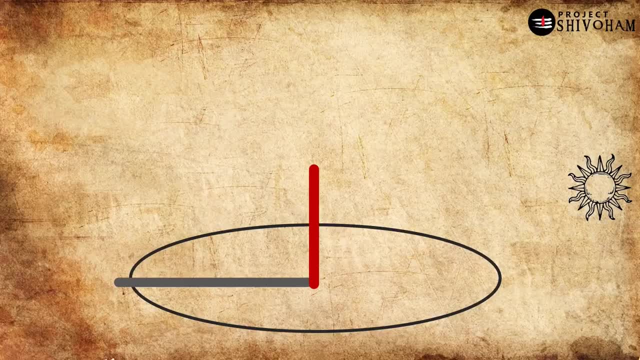 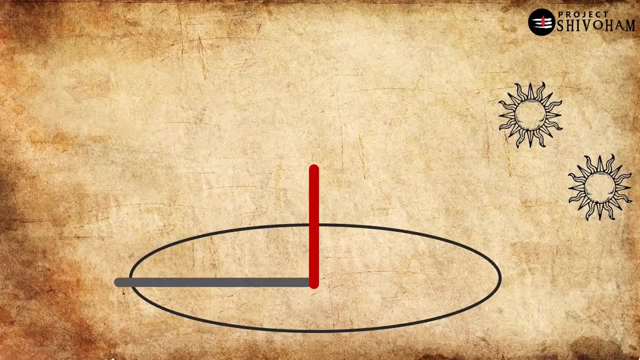 and then draw a circle around the stick like this, and this has to be done before the sunrise. and once sun rises, the shadow of this stick is casted on the opposite direction, so the longest shadow will be in the early morning, so the shadow protrudes out of the circle that was drawn. 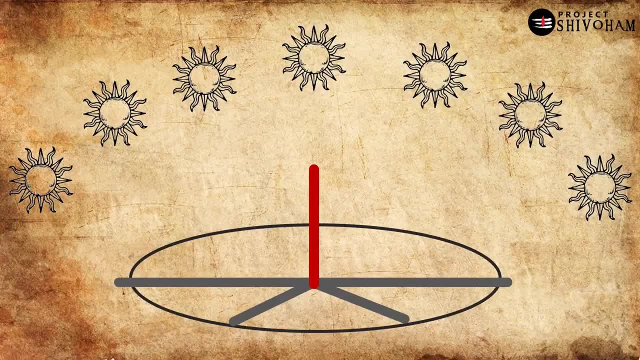 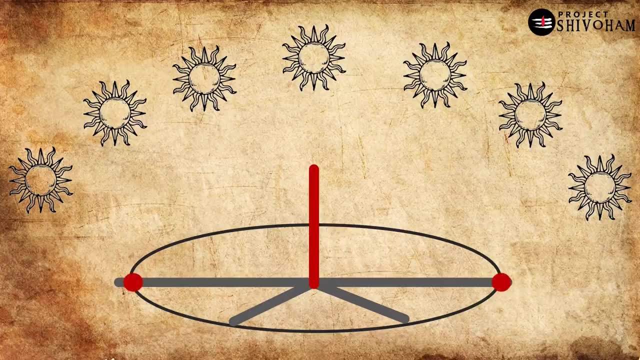 and as the sun progresses over the day, proportionally the shadow reduces and in the evening again it protrudes towards the other end. so these two spots which cross over this circular path, these two points give the east west line. now that we have the east west line, the next step is: 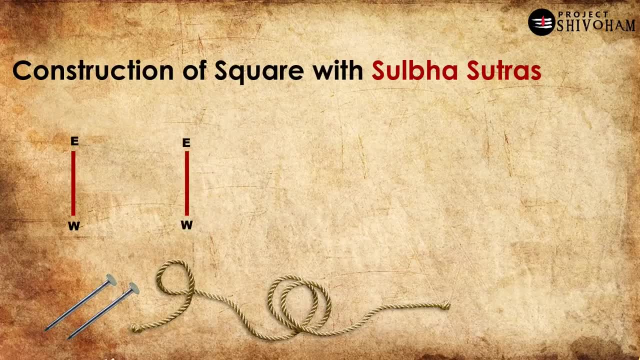 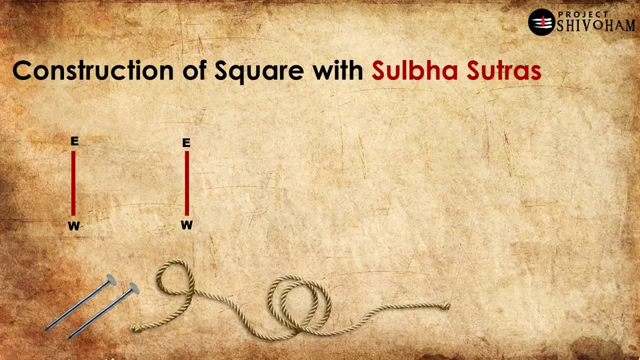 translating directly the process given in sulpa sutras: first take the east west line and draw it to the length of the square that you want. say, for instance, 10 angulas, so ew should be of 10 angulas. then, with that as a diameter, draw a circle again. to draw a circle, like i said, measure 10 angulas. 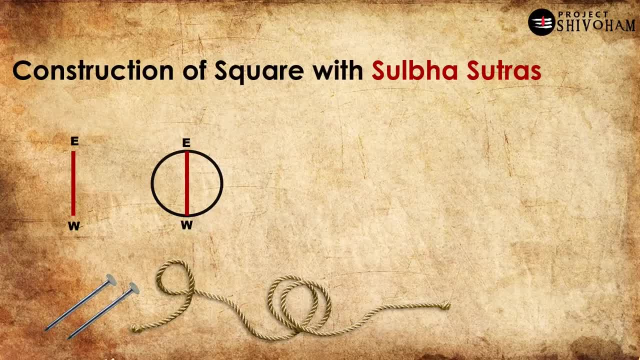 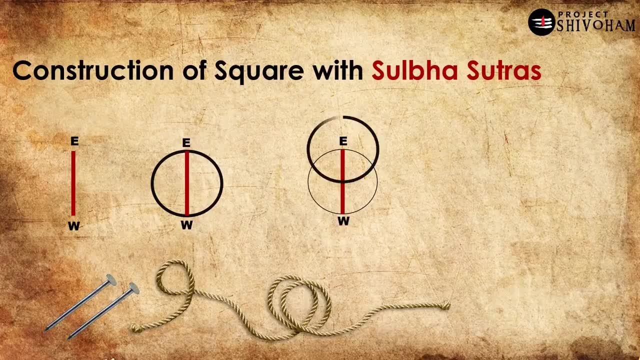 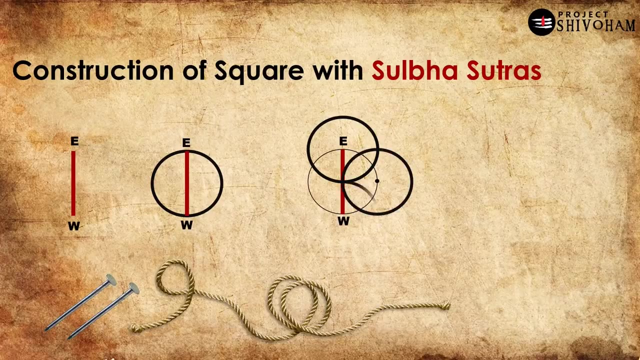 with a rope and with ew as a diameter. draw a circle around it, now taking the same ew as a diameter, with e as a center. draw a circle around it. after that, take a point on the circle, which is: draw a circle around it with the same diameter of ew. repeat this process again, for with w as a center. 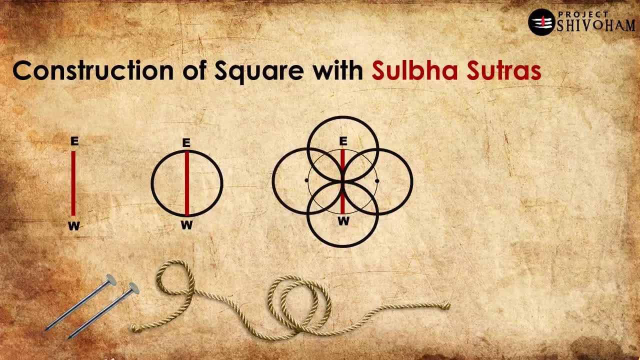 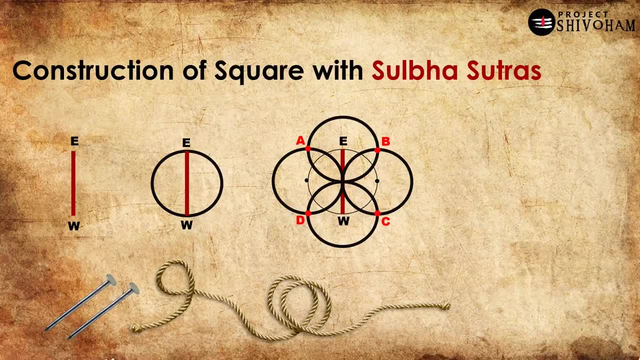 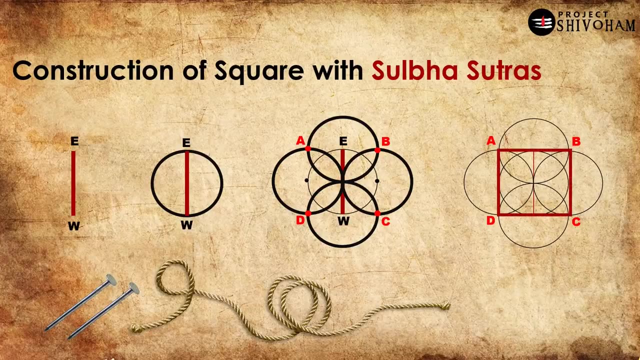 and now, with the opposite point, the second one with the same diameter. so you now have four circles and these four intersection points of these four circles need to be plotted. a, b, c, d. now, joining a, b, c, d gives you a perfect square, with its sides aligned with the four cardinal. 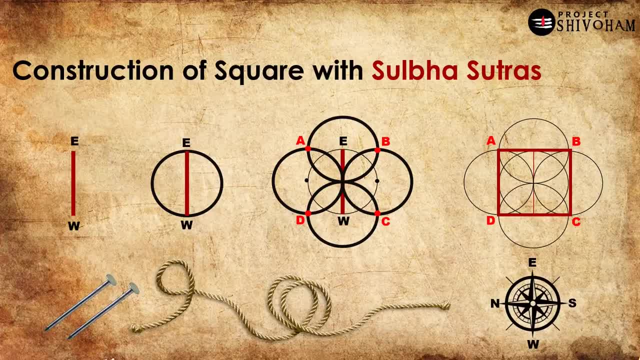 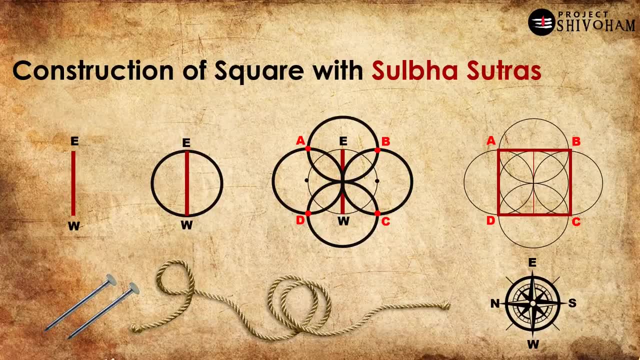 directions and the length that you desire, which here is 10 angulas. so this is how geometry was back then: very primitive, but still precise as well. so once you construct the square on the ground, that forms as the marking for construction of the square, shaped fire altar or the yajna kundam. 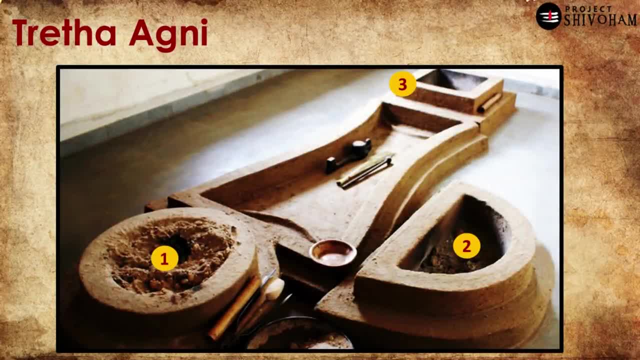 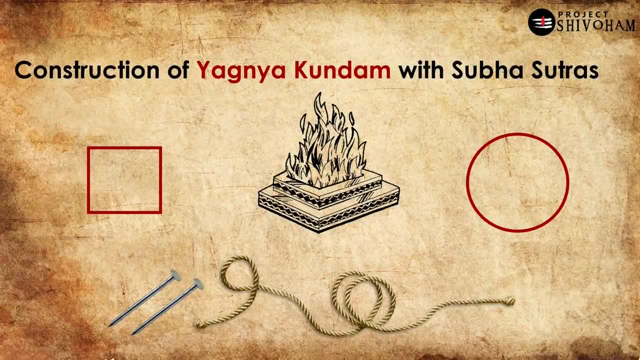 so, coming back to tritagni, where we started, we now have the markings needed for construction of a square shaped fire altar, as you can see in this picture. now they have to construct a circular one which has exactly the same area as the square. so how is that possible? let's see, we cannot talk. 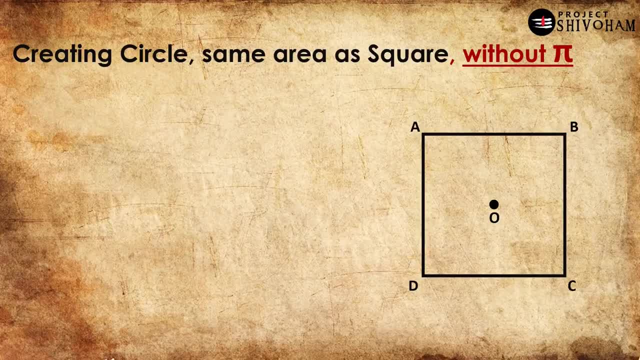 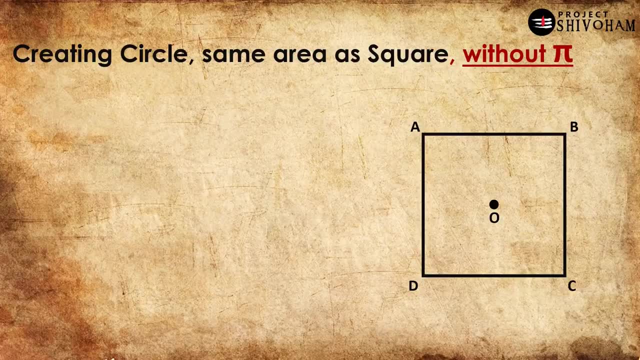 about the circle without pi. but back then the pi was not discovered. yet the credit of pi goes to greeks or, arguably, egyptians- one of these two civilizations- indians don't know about pi during those times. remember we are talking about couple of thousands of years ago. don't just go with. 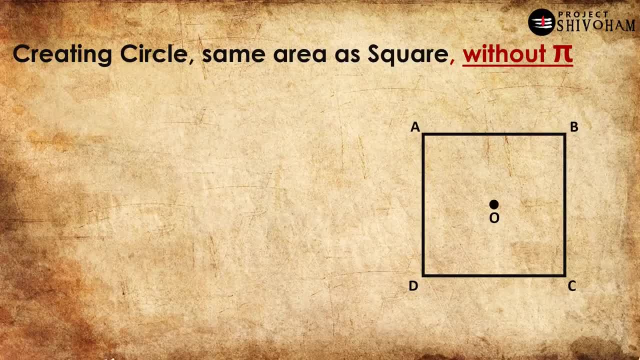 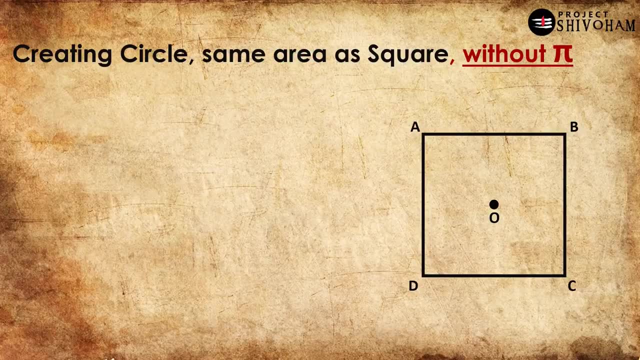 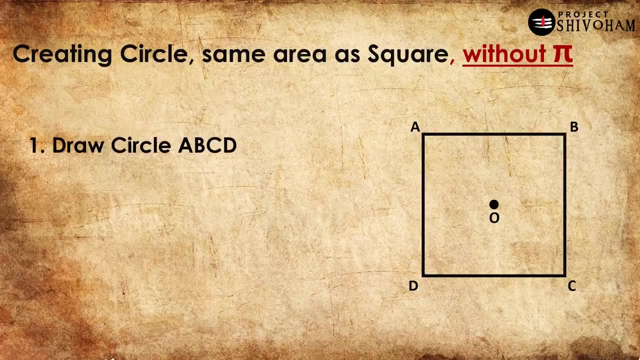 current datings of 500 bc or 1000 bc. it is much, much older than that. so back then pi was not discovered yet. so here is a beautiful postulate given by sulbasutra on how to convert square, which is a circle of exactly the same area, and here is the process given in silver sutras: draw a circle a. 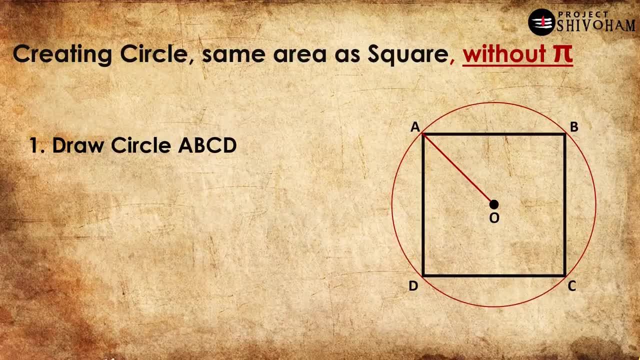 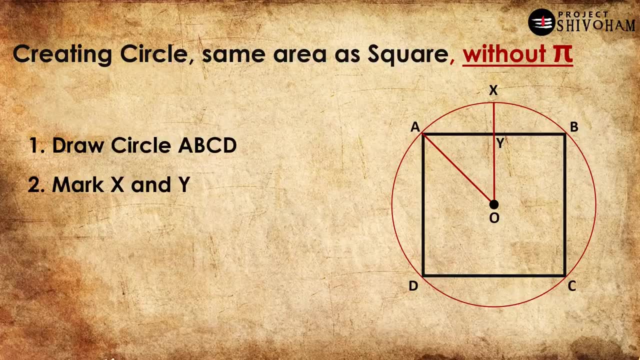 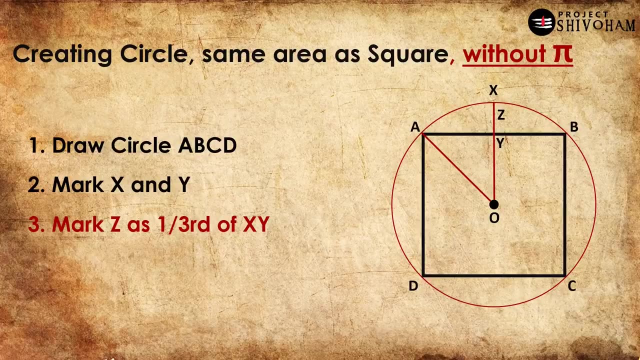 b, c, d and then mark x and y extending o. so we have x and y as part of x and y divided into three parts, so that mark z as one third of x- y, so y- z is one third and z- x is two thirds of x- y. 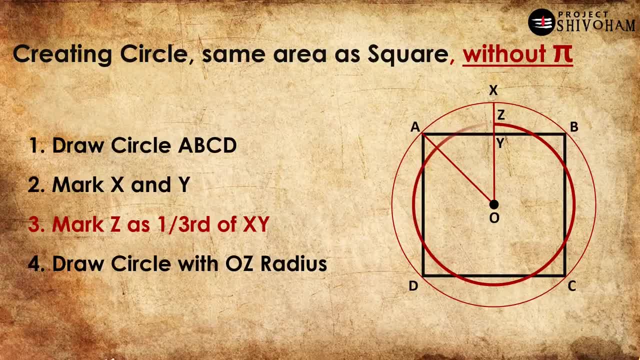 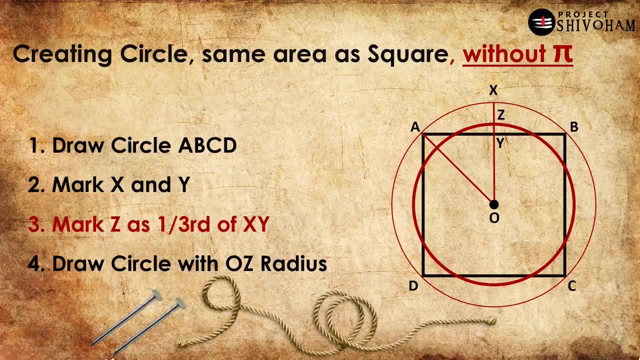 and then mark x and y, and then mark x and y is one third of x- y, and then mark x and y is one third of x- y. so this is the most important thing. so, finally, draw a circle with o- z as the radius. so this is the most important thing, with o- z as the radius, the circle that you're drawing here. 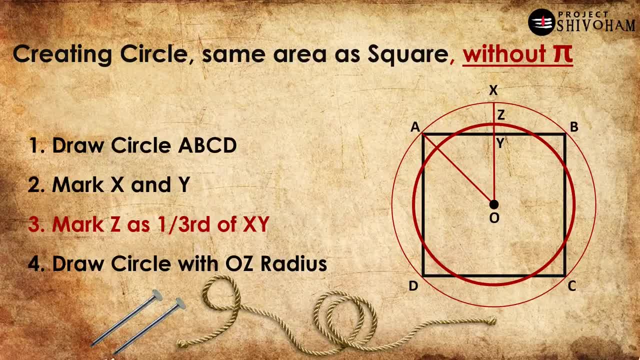 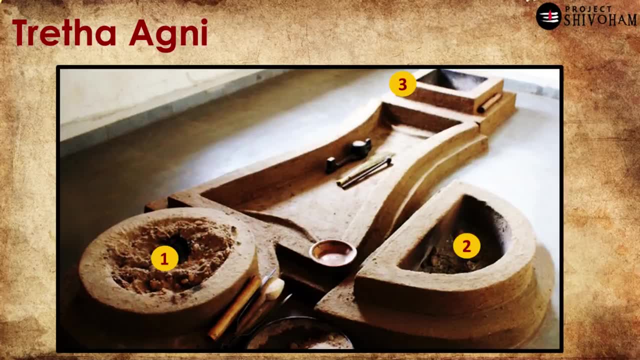 is exactly of the same area as the square. a, b, c, d, so this was a postulate that was given, which can be geometrically proved today as well. if you want, try it out. it's really great to see how organically the circular fire altar as well, which is exactly of the same area as the square. like this there are. 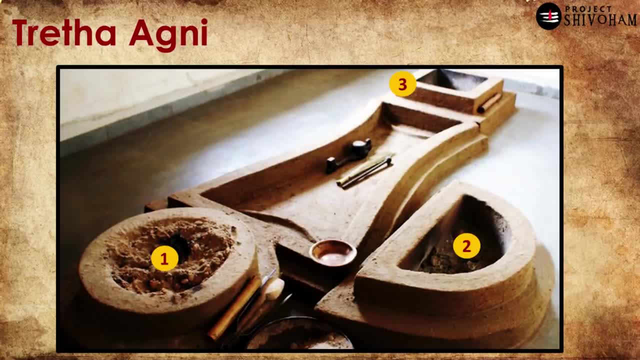 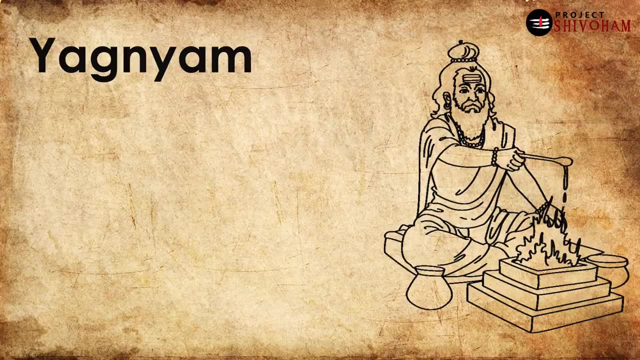 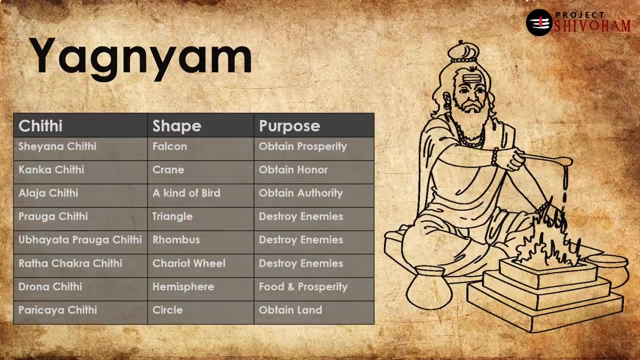 many, many geometrical principles explained in sulva sutras. but for now, let's move on. these fire altars are called as chiti in samskritam, and depending on the intent of the yajnam, the shape of the chiti varies. for instance, to obtain prosperity, a falcon shaped chiti is constructed. 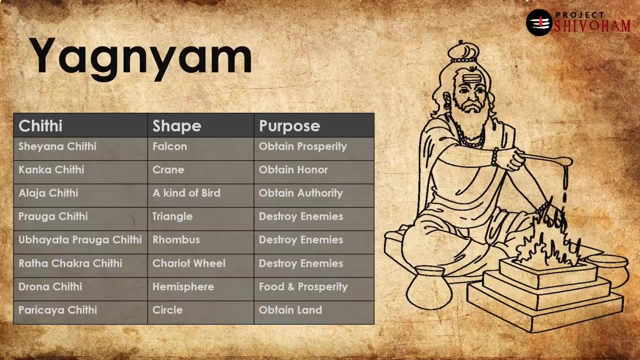 to destroy the enemies in war, a triangular or rhombus kind of a chiti is constructed, and to pray for food and prosperity of the kingdom, a hemisphere shape of chiti is constructed. so depends on the intent. the process given for the yajnam is different, and so is the shape of the 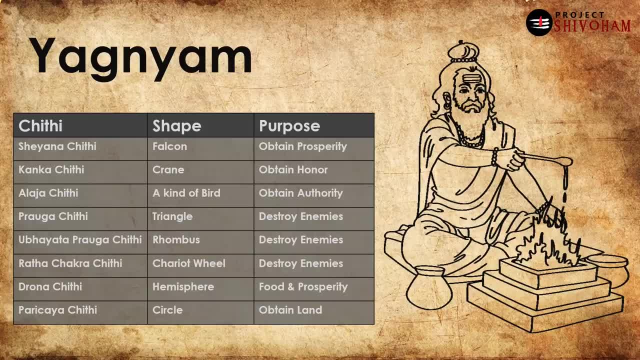 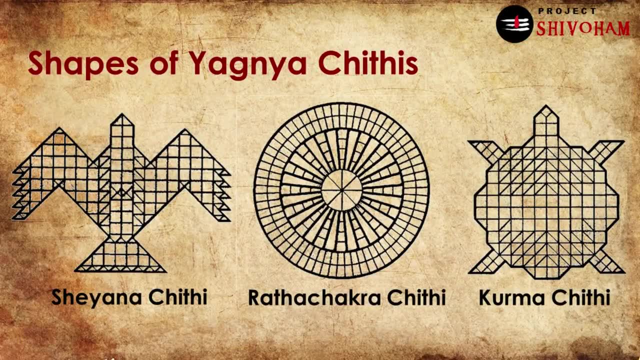 chiti. this is very important because this has defined the dynamics of vedic geometry. so these chitis are not just made out of mud, they are made out of brick arrangements and this is how the blueprints of couple of chitis, like shana chiti, rada chakra chiti and kurma chiti are. so this is 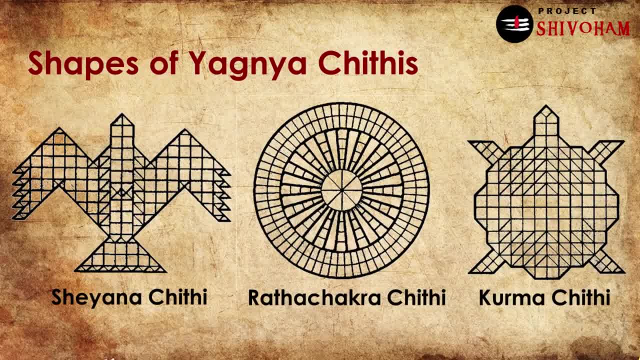 from kalpa, which ascribes to yazoor vedham. so here the most important aspect of the yajna is, that is, the bricks need to be baked according to the dimensions given here, and that needs to fit exactly in the shape of the chitti. If you observe the shapes of the bricks, they 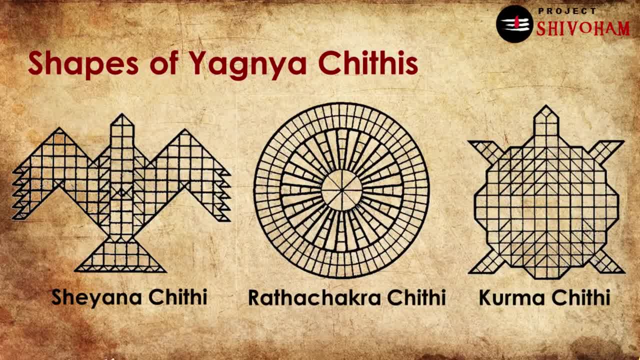 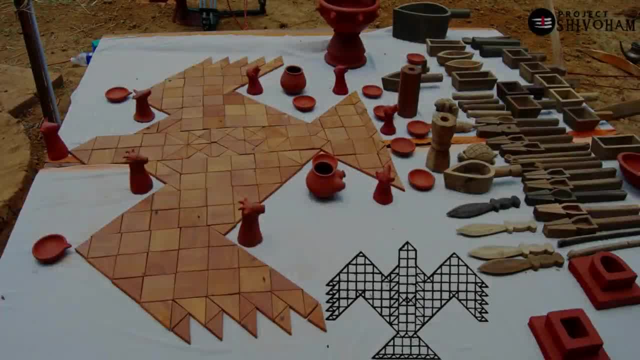 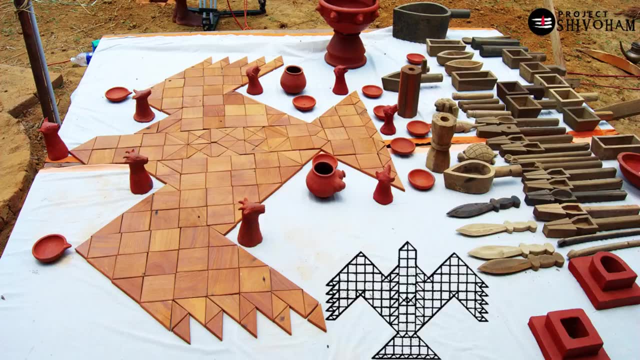 are squares, rectangles, triangles, rhombus trapezium. So here is where the Vedic geometry gets totally into another level. Here is an example of Sheyana Chitti, which shows a miniature model about how the bricks need to be cut. Observe the tiles, how they are shaped. They. 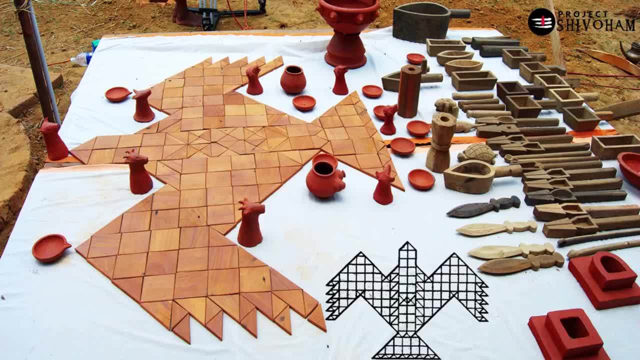 are right angle triangles, isosceles triangles, squares, rectangles, everything stacked up to form the shape of a Garuda or a falcon, which is an exact replica of the blueprint that you are seeing here down below, And all the wooden equipments that you are seeing. 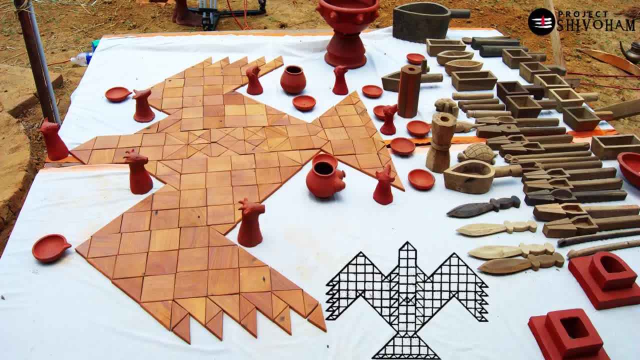 around. it are the ones that are needed for executing a Yajnam. The interesting part here is now: what is the geometry behind cutting and baking of these bricks? That gives us some incredible facts about Vedic geometry. Let's see what they are. 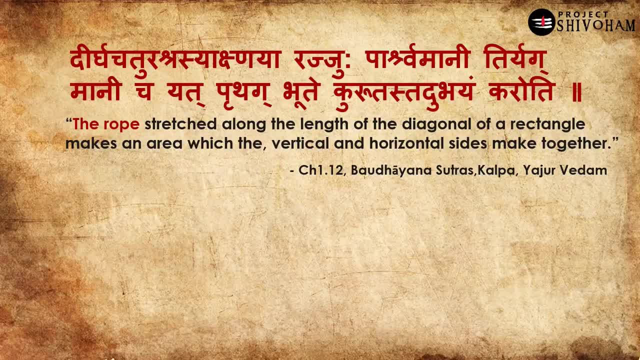 To calculate the geometry of the bricks. we need to calculate the geometry of the bricks, To calculate the dimensions of these bricks based on the shapes. there are a lot of formulas or principles given in Sulva Sutras. Here I just picked up one example which is very 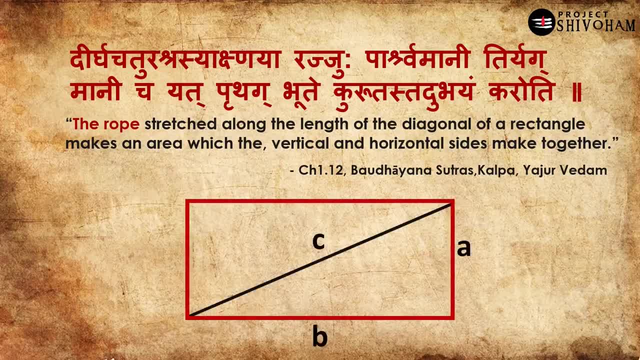 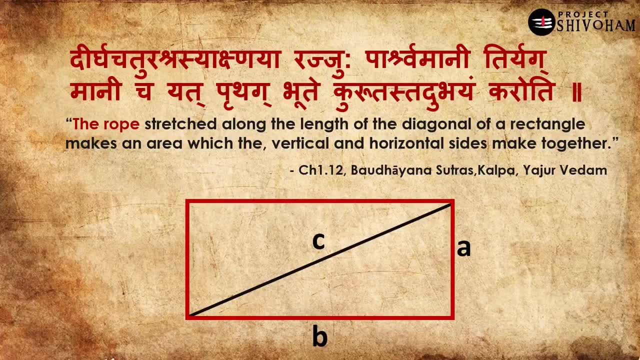 relevant to you and me, based on what we learned in our school, And this is how it reads: Dhirgha chatra srayakshanya rajyahu pashvamani triyam manicha yatak prudhak bhute kurutastu. 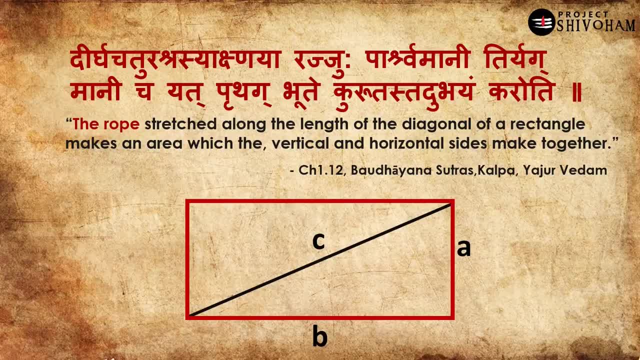 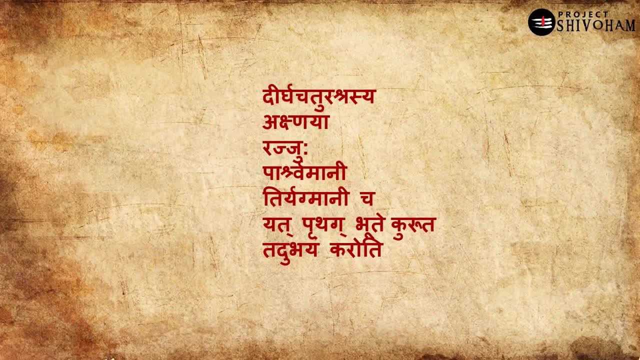 dabhayam karuti. Basically it talks about a rectangle, but let's break it down word by word to understand the exact meaning of it. Dhirgha chatra sraya, which is a rectangle. akshanya means diagonal. rajyahu here means: 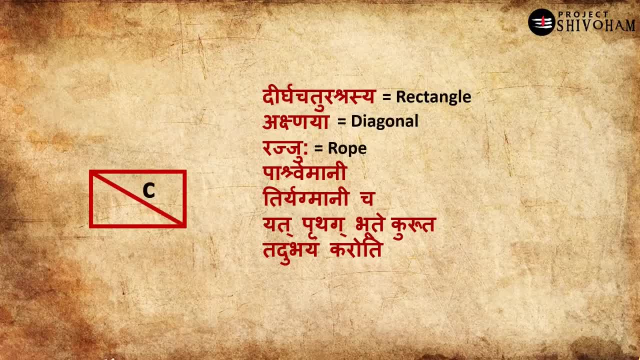 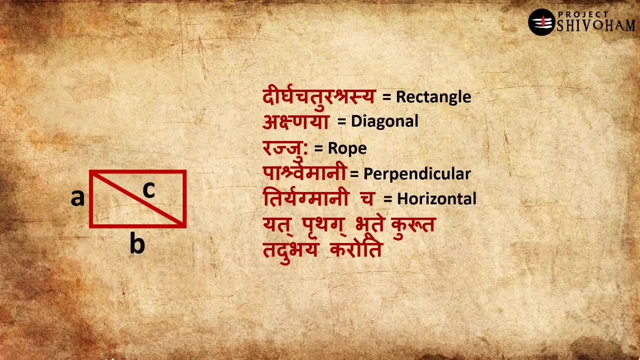 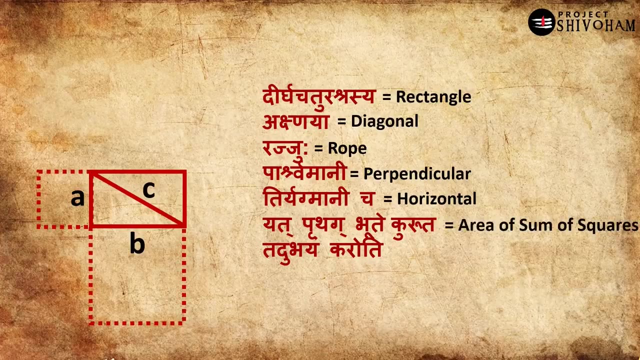 rope for measurement. Let's put that aside. Pashvamani means perpendicular or straight, and triyam manicha, which is horizontal, yatak prudhak bhute kuruta, which means area of the sum of the squares, dadubhayam karuti, which equals the area of diagonal. So basically, 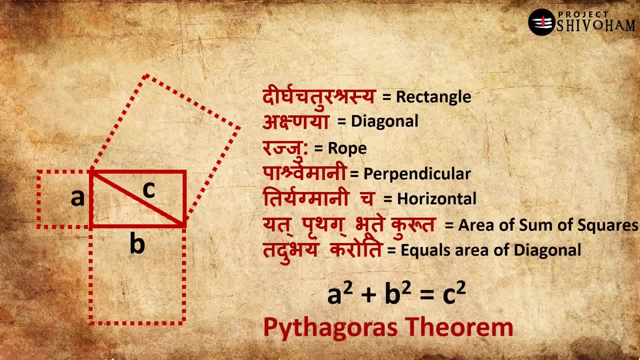 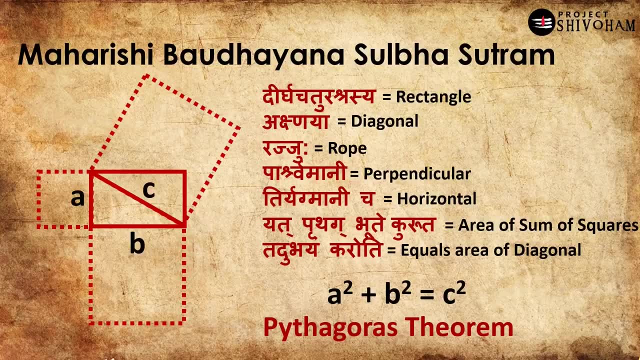 what it says is: The area made by the horizontal and the vertical lines of a rectangle is equal to the area made by the diagonal. This is called as Pythagoras theorem in today's world, but is actually written by Mahashree Baudhayana, who is conservatively dated as 800 BC. But again, like I said, 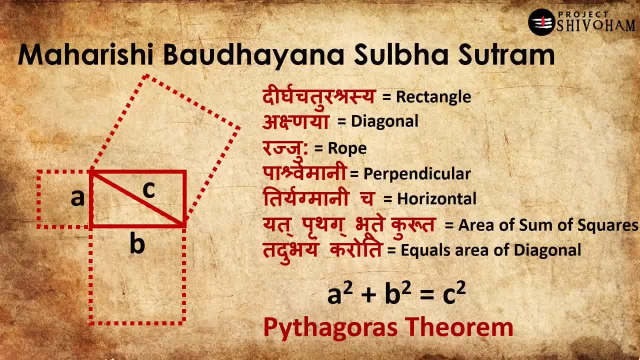 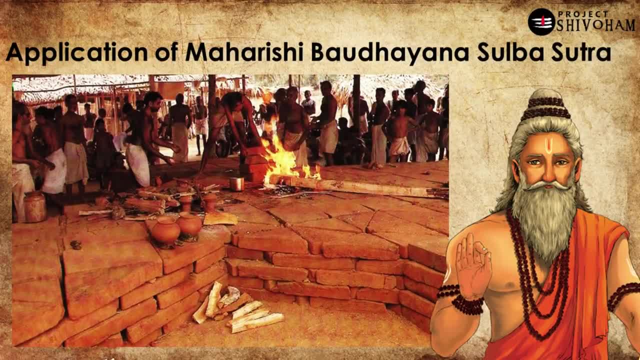 shayana chitti, which is in the form of a garuda or a falcon. Look at the size and the shape of the bricks. They are in triangular forms, stacked up into five layers. Now the geometry behind cutting and baking of this bricks is fully based. 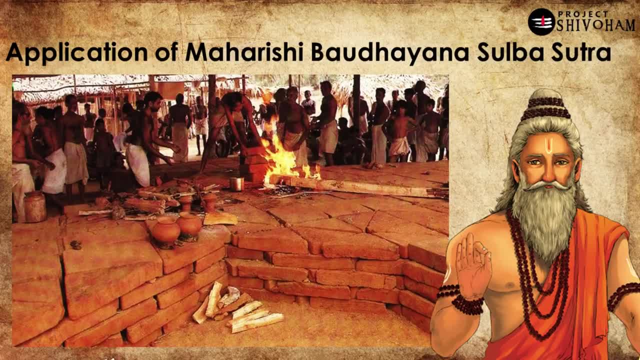 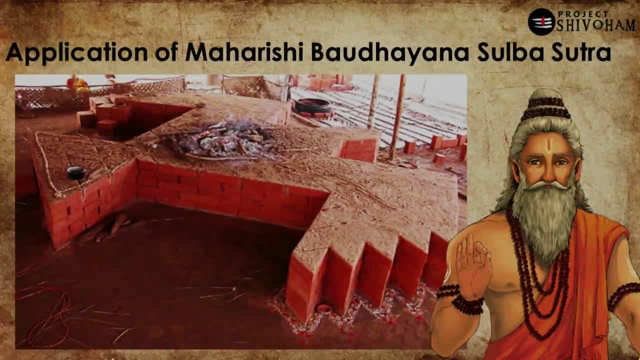 on sulbha sutras even today. And the so called Pythagoras theorem, which we just saw, is just one of the many geometrical principles given by Maharishi Baudhayana. If you observe it from this direction, you can see clearly how the entire fire 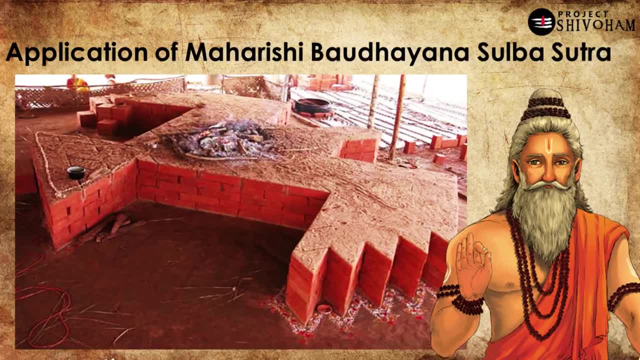 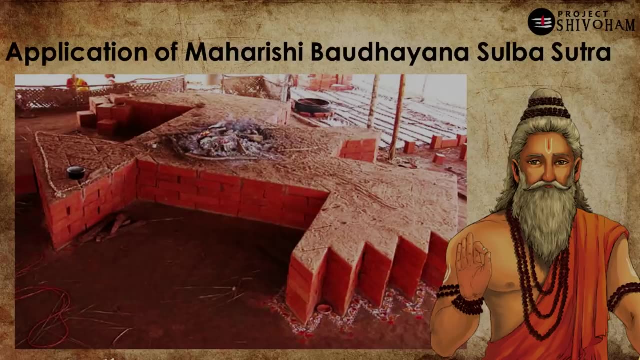 altar is in the shape of a falcon, like we have seen in the blueprint. So on top of this, the entire yajnam will be performed. Now, because of these five layers, the complexity behind the geometrical construction of these bricks even gets multiplied. It takes to a level even above. Let's see what it is. 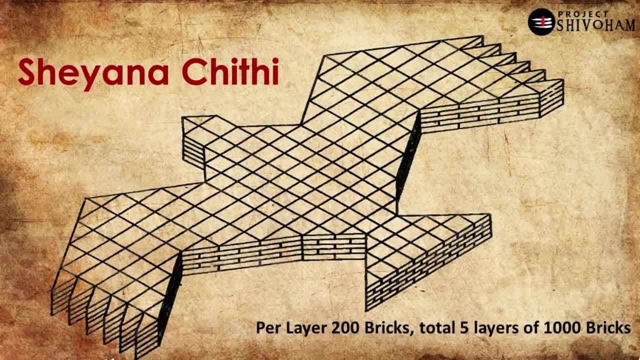 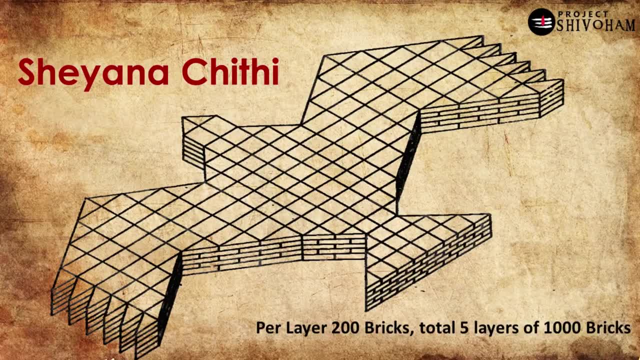 Let's take the isometric view of the blueprint of shayana chitti Here. if you see, it has five layers, all exactly in the same shape, and there is an additional constraint that is imposed by the sulbha sutras that there should be only five layers in this one and each layer can have only 200 bricks. 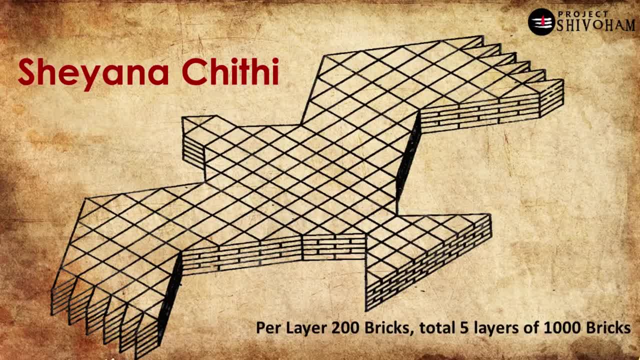 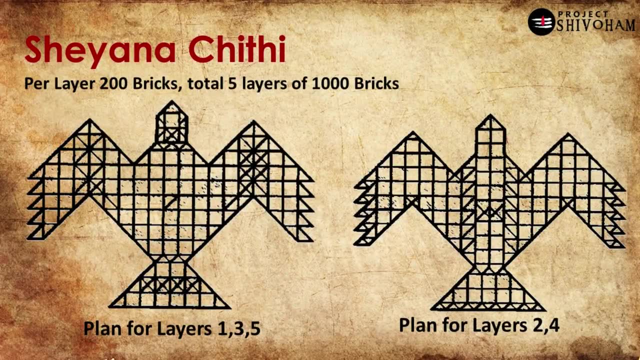 and in five layers. so that is 1,000 bricks. So you have to finish this entire construction of shayana chitti in just 1,000 bricks, with exactly 200 bricks per layer. If you are thinking that's complex, it's still not done yet. The five layers: 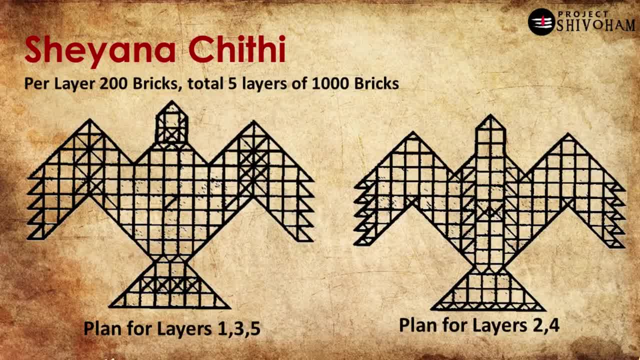 of the shayana chitti, the layout for 1,, 3 and 5, the odd numbers layout is different from that of the even numbers. So, towards left, what you're seeing here is the layout for the odd numbers and the right side is for the even numbers. So 200 bricks, two layouts, five layers, no. 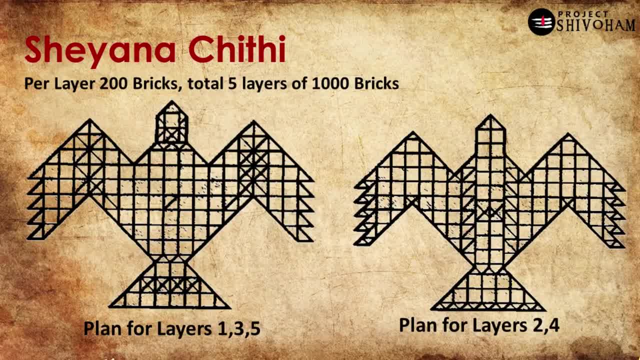 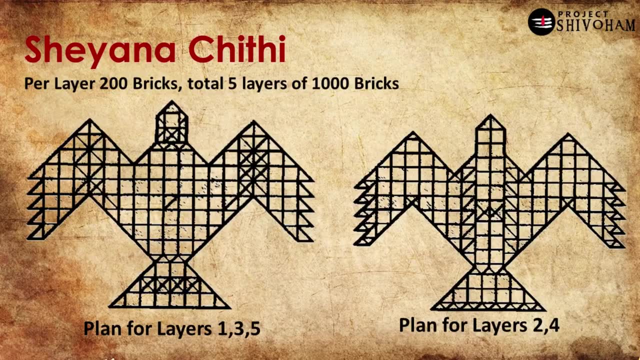 scale, no equipment, nothing. In a very primitive way the entire geometry has been executed and this is just an example to show how complex problems sulbha sutras dealt with, and this is the reason why sulbha sutras are considered as world's oldest applied geometry. and after sulbha sutras we have the 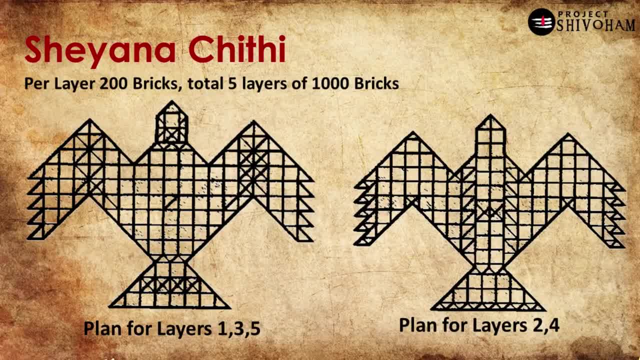 Euclidean geometry that came in 300 BC. 99 percent of Indians today are not aware of Sulbha sutras. Just for one reason: we don't care about our own history and heritage. Talking of history here is a bit more about the Pythagoras. 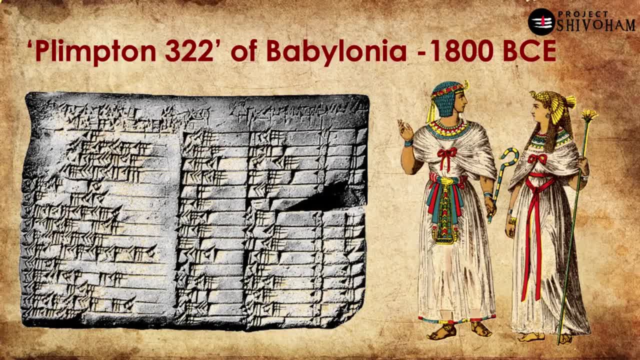 theorem, The Pythagoras theorem, or the Pythagoras triplets, which satisfy the Pythagoras theorem, are first found in Babylon, which is modern-day Iraq, inscripted on a stone tablet called as Plimpton 322- that's the code name given to it. 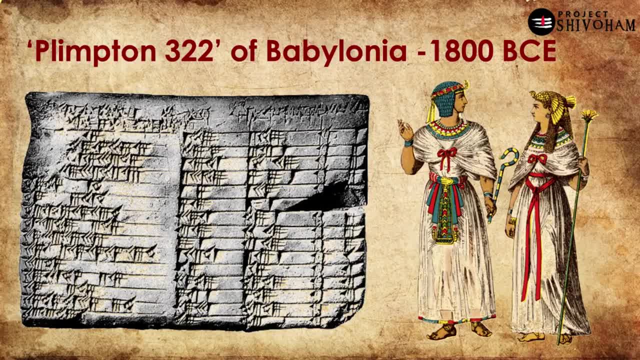 into the tablet, but it is dated to 1800 bc, which is first found in babylon. so it is almost 1300 years before pythagoras discovered the pythagoras theorem. and this is the tablet. what you're seeing on the screen. the pythagorean triplets are carved into three columns, so these are like three numbers. 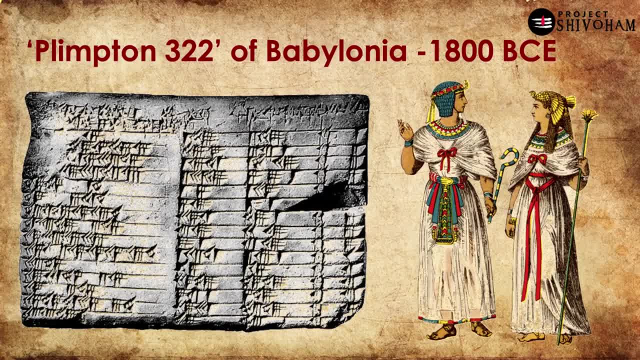 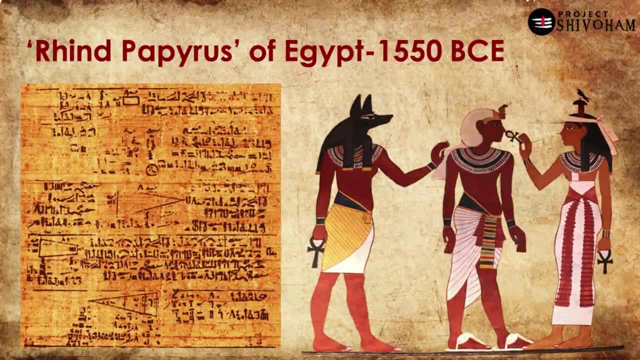 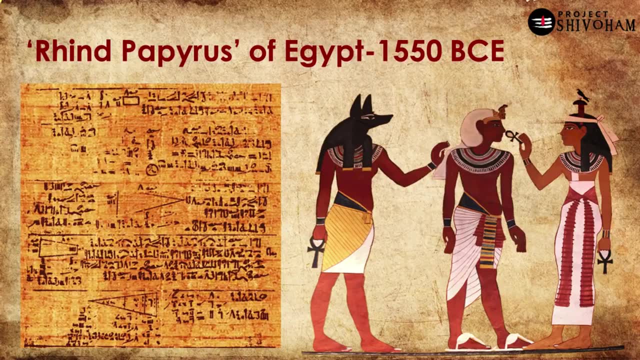 which satisfy the pythagoras rule, and these combinations of numbers are very crucial and they have a lot of applications. you can search for yourself. another ancient source of the pythagoras triplets comes from egypt, a mathematical document called rin papyrus, which is a mathematical 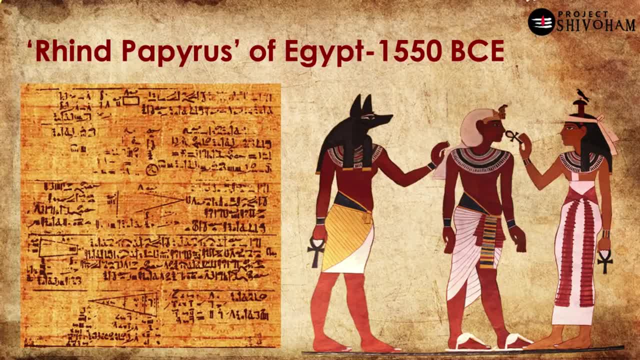 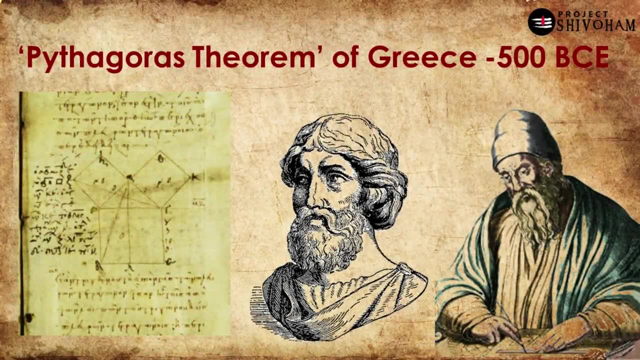 worksheet of the ancient egyptians. apparently it also has the pythagorean triplets calculated, and this is almost dated to approximately 1500 bc- and, as you know, egyptians are very famous for their triangular structures. and finally, from the greeks, in 500 bc, pythagoras is the one who generalized the property of a right angle. that 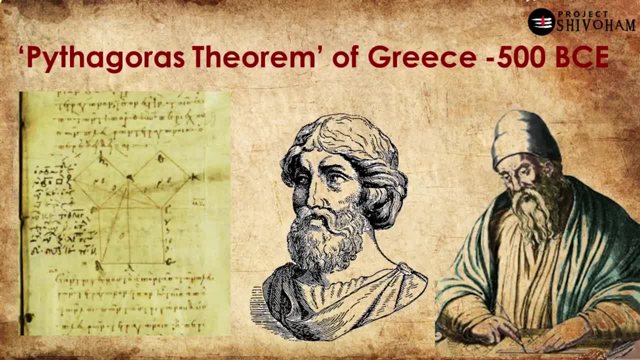 the base square plus side square is equal to hypotenuse square. however, the pythagoras theorem- what we know today- is given to us by euclid, a greek mathematician, 200 years later after pythagoras. he's the one who is documented and that's the manuscript, what you're seeing here. 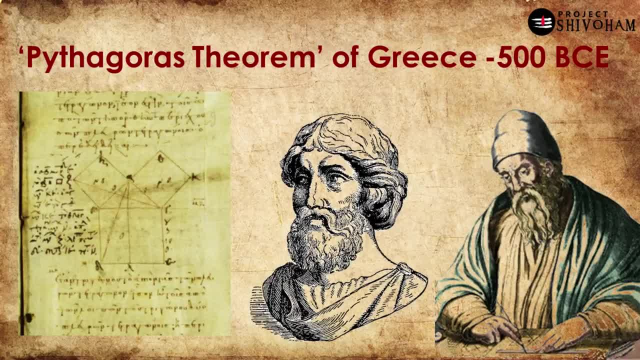 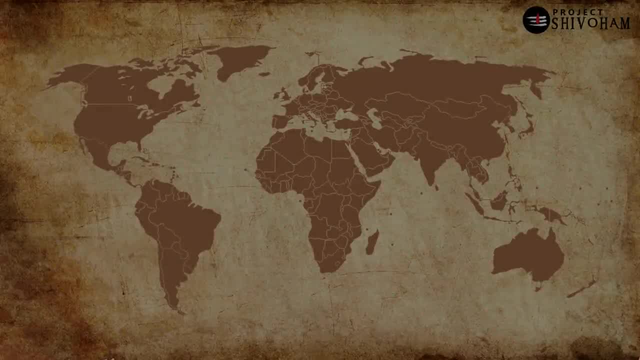 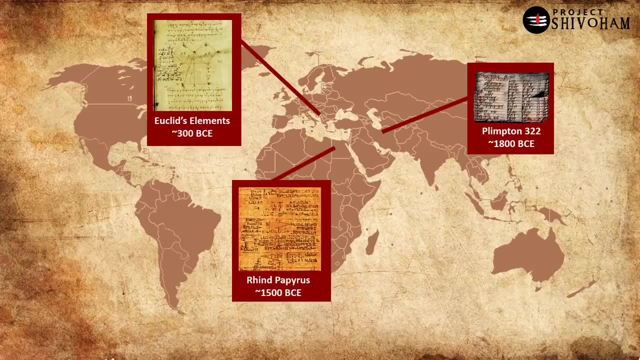 it is possibly a copy of euclid's original, or could be a recopy of a latin version, but nonetheless it's a manuscript explaining about the pythagoras theorem. now, if we take a macro, look, it is babylonians in the 1800 bc, egyptians in the 1500 bc and greeks in. 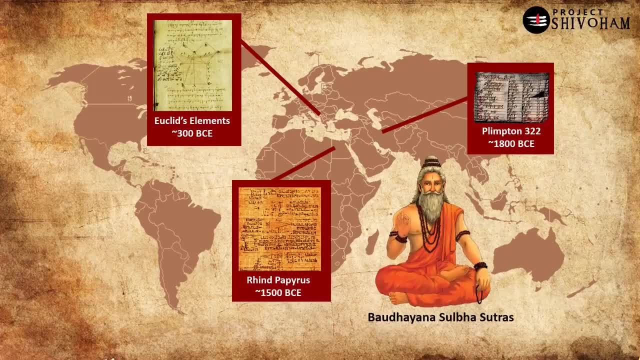 approximately 300 to 500 bc, and maharshi baudhaina, who is again conservatively placed at 800 bc, gave the formula much before it is generalized by pythagoras. it is not just about the antiquity, but also about the continuity. since many, many thousands of years, the sulba sutras have been 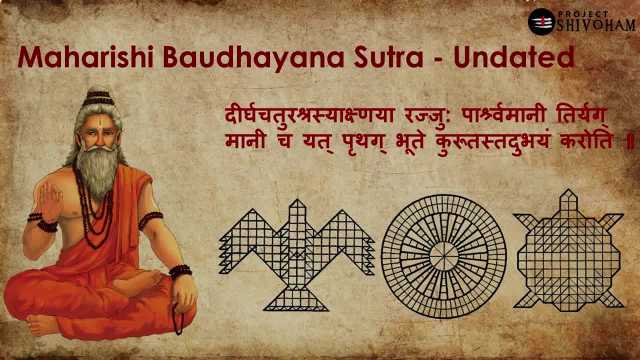 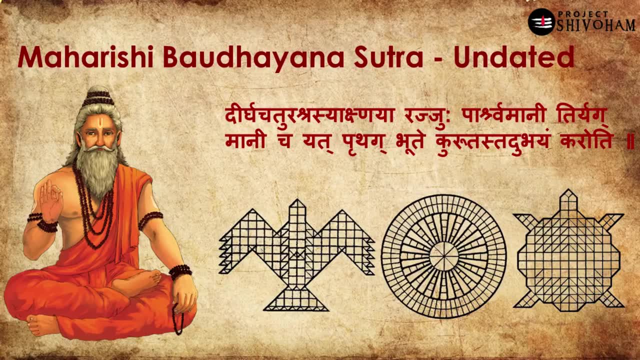 defining the way a yajnam needs to be organized, and till today it is in practice, such as the. yajnam is the rich heritage when it comes to vedic geometry, yet there is a high probability that most of you would have never heard of it. i just took this one as an example so that most of us 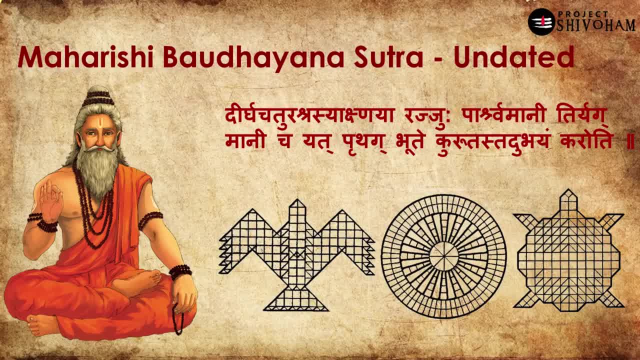 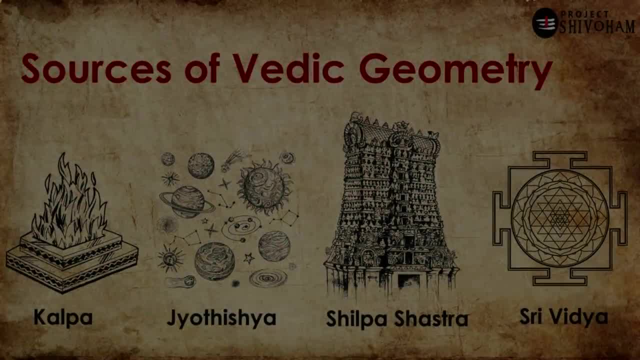 can connect and understand. but like this, there are baudhaina, apastamba, manava, kathayana sulba sutras talking about the geometrical principles. so that's about the geometrical principles in kalpa, and now let's move on to jyotishya. 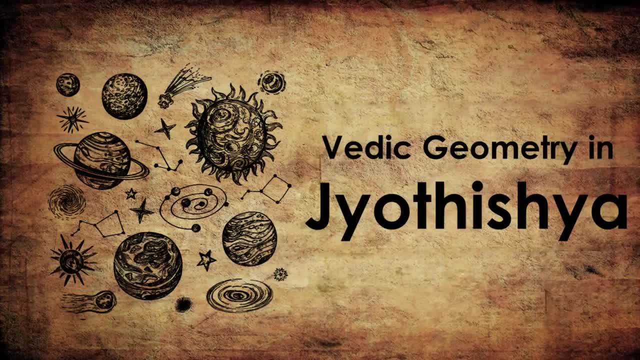 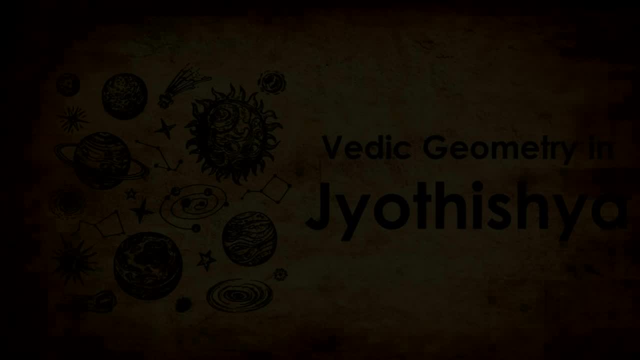 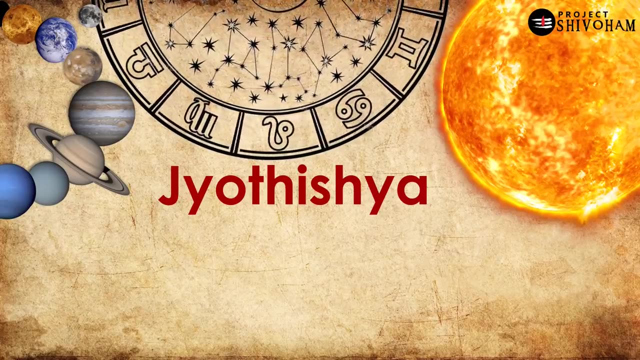 jyotishya, misunderstandings, misconceptions, pseudoscience, what not? it is totally entangled in a lot of preconceived notions. and allow me to set the record straight here: there is astrology, which deals mostly with the cultural element of predicting the future, and there is astronomy, which is the study of the celestial bodies. 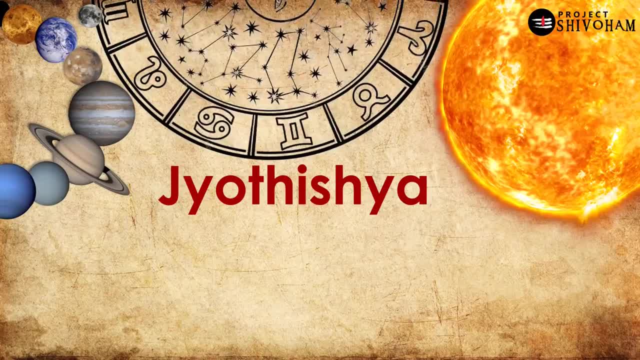 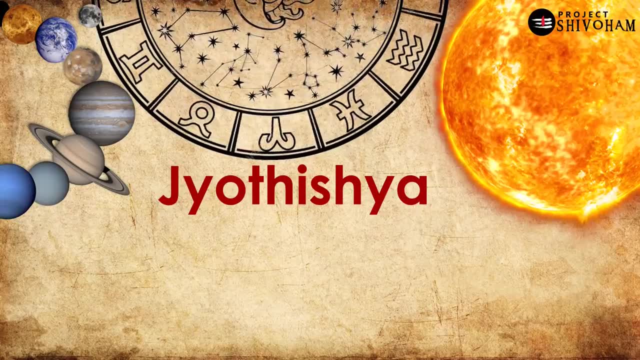 now getting straight to the point: is astrology or that future prediction business? is that scientific or not? well, the answer is: i don't know, and i'm not bothered either. let us take a worst case assumption that it is totally a pseudoscience. but the fact of the matter is. 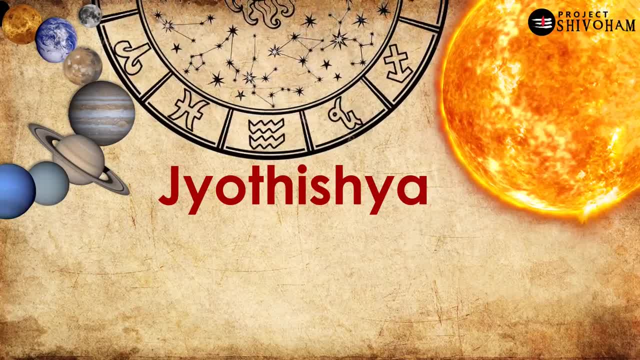 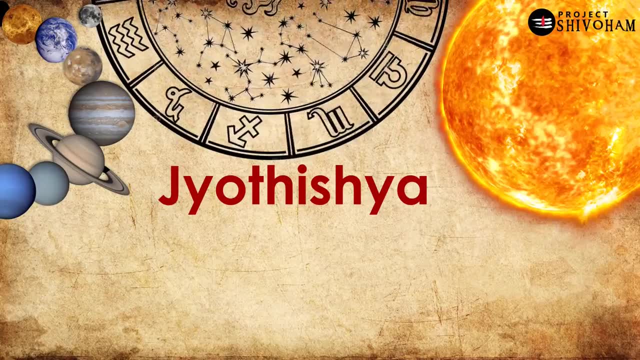 that astrology is not a pseudoscience. because astrology is not a pseudoscience, because astrology is not a pseudoscience because of astrology, astronomy existed in india. historically there have been a belief that the planetary positions impact people's lives. now again, i repeat, we are not at all discussing about that aspect here and we are least interested about 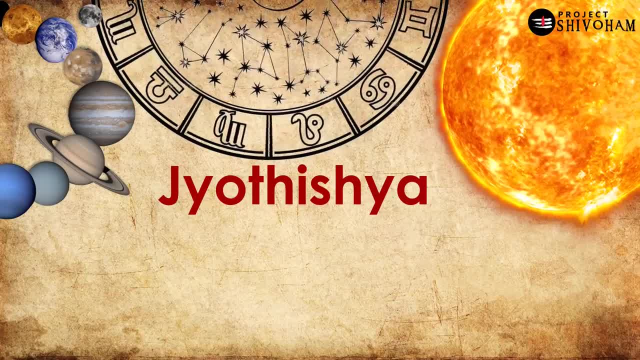 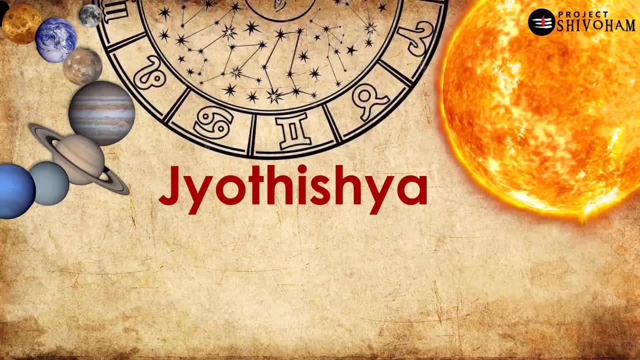 that what we are rather interested is in order to compute the planetary positions. jyotishya gave birth to incredible fields of mathematics, and this is not a joke, or i'm just trying to brew a conspiracy here. if at all there is any branch of knowledge that is highly misused and highly misinterested, then it is jyotishya. 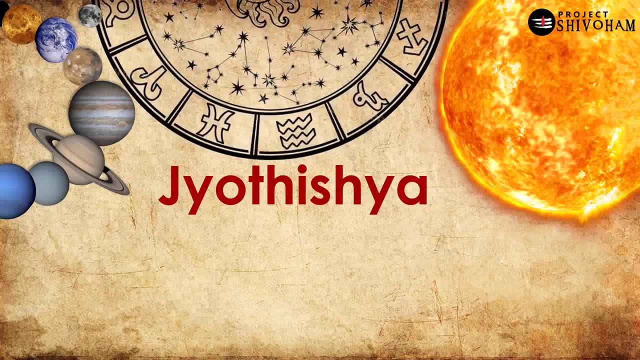 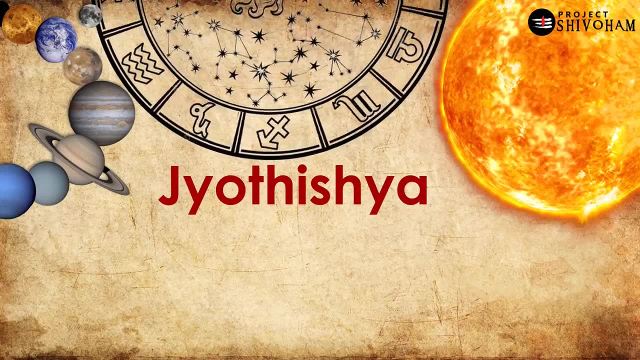 misused because of one set of people who commercialize this entire jyotishya shastra, and misunderstood because of another set of people who don't know a thing about it but just outright say that it's a pseudoscience. now let's forget about these two highly polarized versions. let's 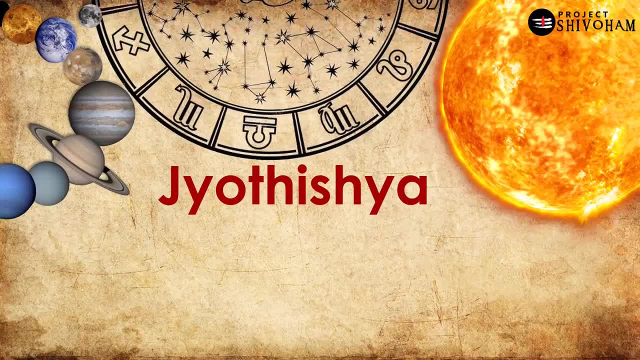 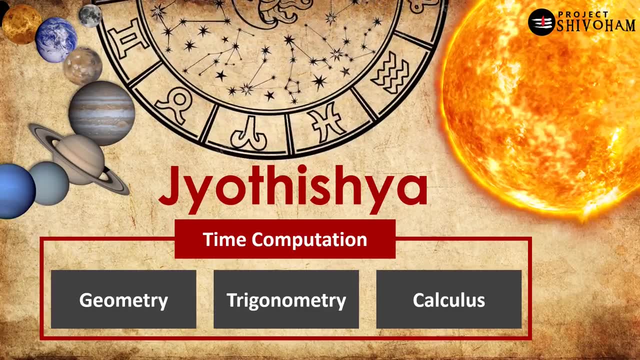 try to find out what is in the middle with respect to geometry and, at large, with mathematics. time computation, it is the heart and soul of jyotishya. calculating the planetary positions to the minute is of top-notch importance, and to do so the ancient indian astronomers 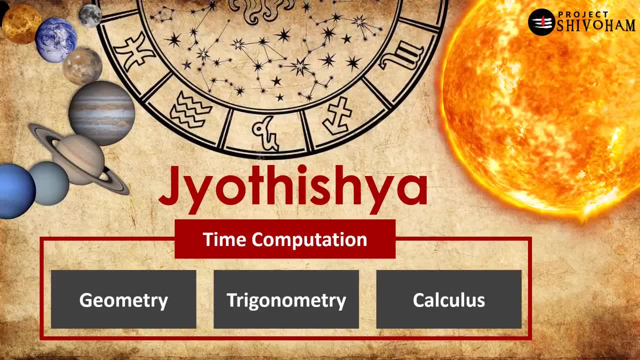 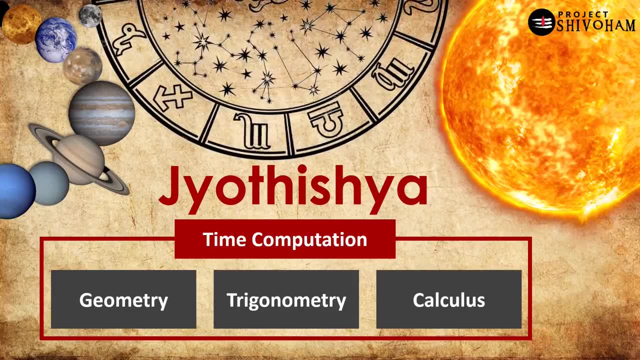 and mathematicians developed a fleet of mathematical concepts in these three areas of geometry, trigonometry and calculus. let me put all these four blocks in a simple perspective. the time computation is of the top-notch importance and, in order to do that, the rate of change of planetary 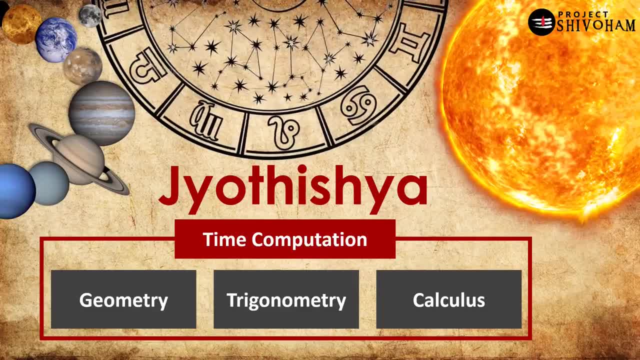 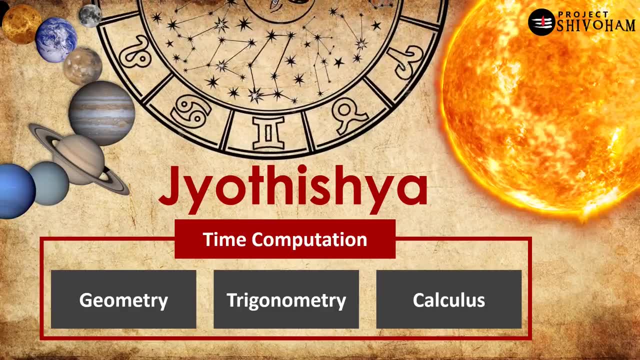 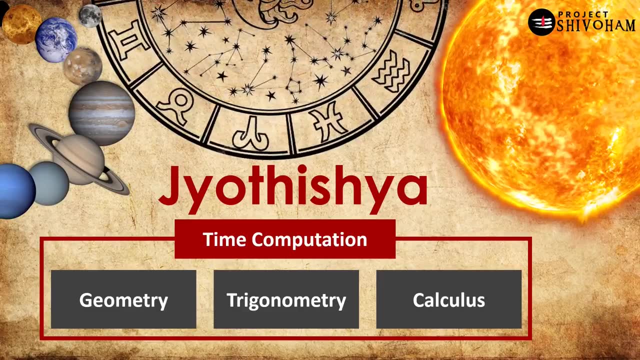 motion is also an integral part of it. because of that, calculus originated and is a precursor to calculus. to calculate the ratio of observations of different planets, trigonometry as well took birth, and in order to construct the astronomical equipments, geometry as well thrived as part of jyotishya. these three topics are very much intertwined with each other. 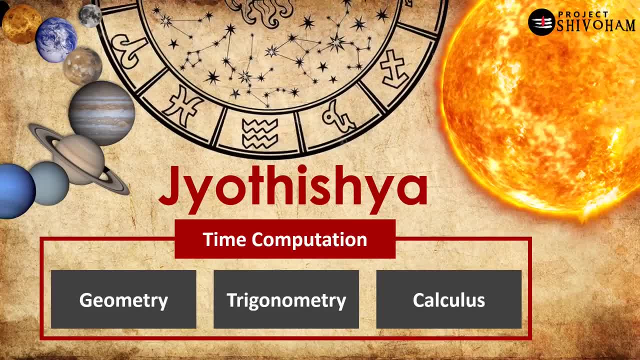 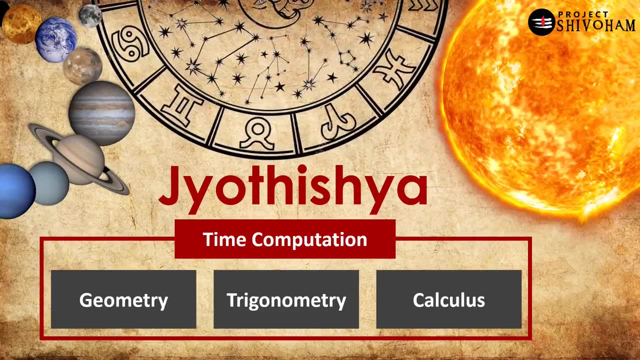 and it is difficult to explain one and leave the rest out. we are planning for a separate detailed documentary on jyotishya, but for now i'll try my best to cover only the geometry aspect of it. maybe i have to repeat myself as well, not saying indians founded all these branches of mathematics. 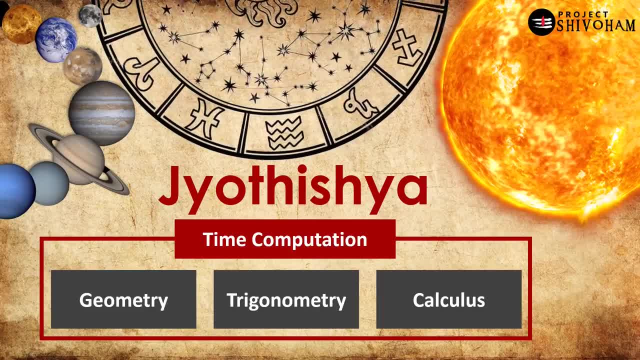 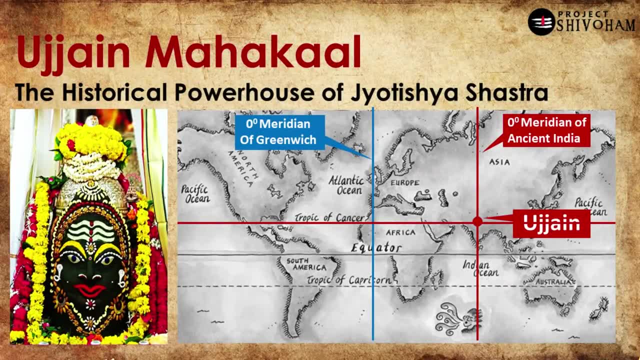 i'm saying there are significant contributions that came in from india for each of these fields which many of the people are not aware. hope i'm clear now. speaking of jyotishya, jyotishya is the most important place in india for two main reasons. number one: it is positioned. 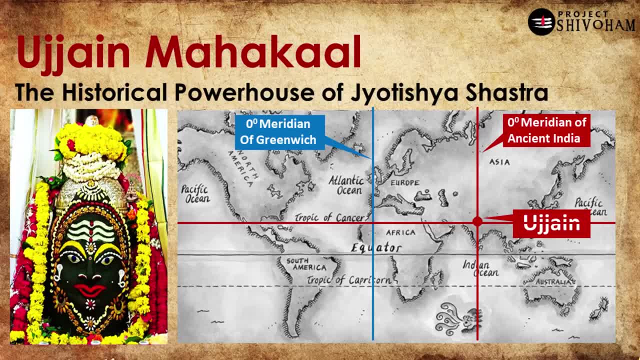 right on the tropic of cancer and for many, many centuries the prime meridian of india used to cut through ujjain, as you're seeing it here, so counting of the day starts from ujjain, as per ancient indian traditions. however, the british- after the colonization in 1884 they kind of consolidated- 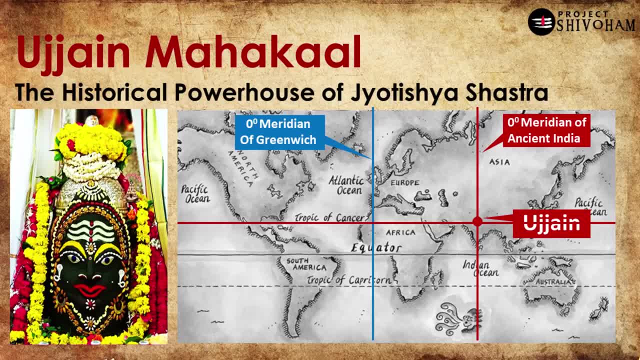 all the meridians across the world where people are having their own prime meridians and moved it to greenwich. otherwise, historically, the meridians were the most important meridians in india and jyotishya is the place where time computation of a day starts. second thing: historically, ujjain produced 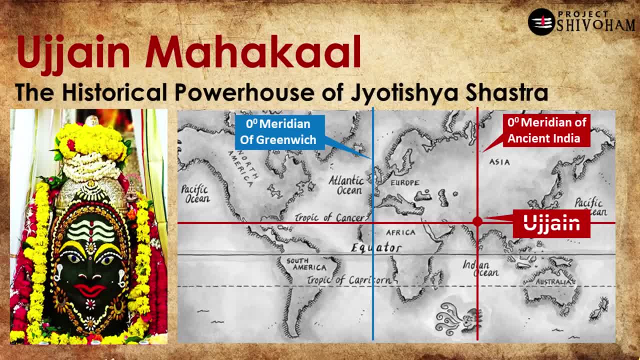 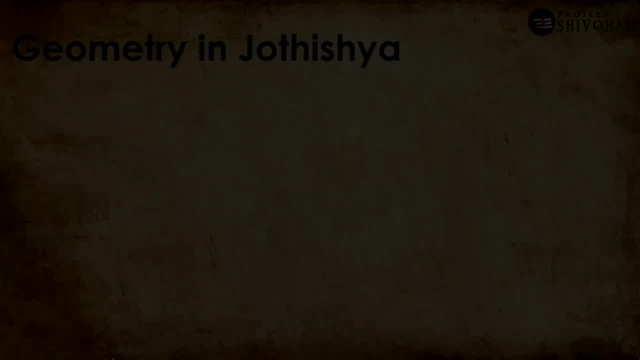 a lot of astronomers and mathematicians who contributed greatly to indian mathematics, and here lord shiva is worshipped as mahakal, which means the lord of time and death. coming to geometry in jyotisha, where all it played its part. here is it that follows. it is used. 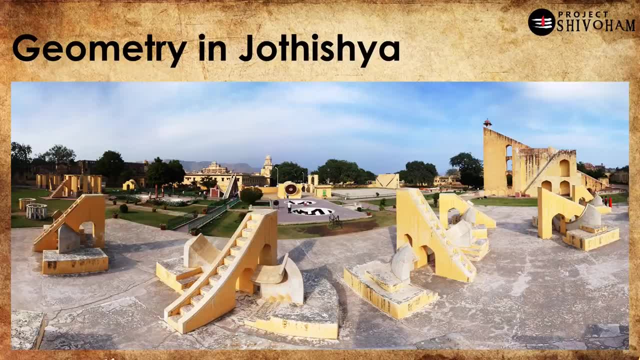 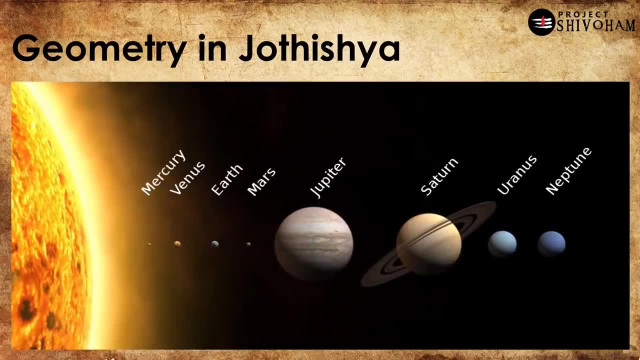 in construction of these astronomical observatories. what you're seeing? different kinds of structures for different purposes, which we have in places like jaipur and ujjain. the next. it also played its part in calculating the radiuses of different planets and also its role in trigonometrical observations to calculate the relative positions of the planets. 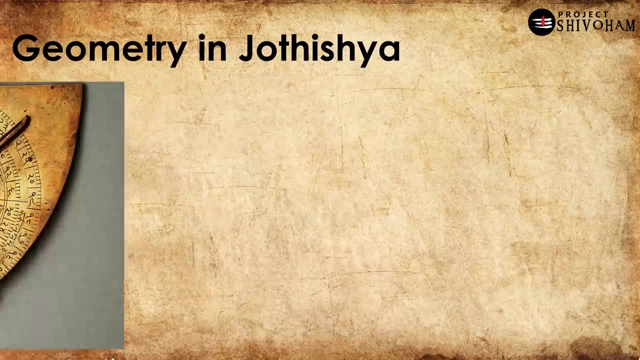 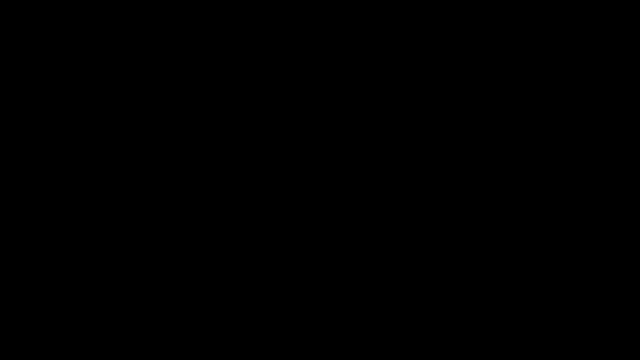 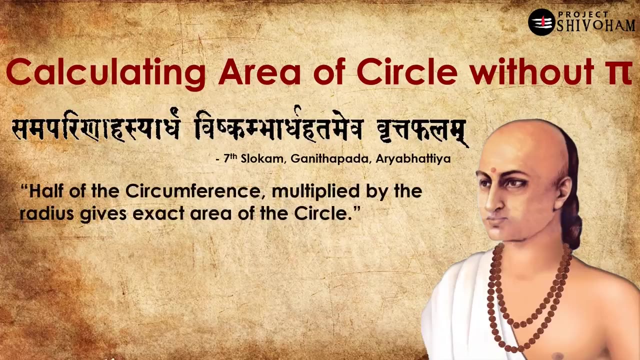 and also in construction of certain astronomical equipments like astrolabes- what you're seeing here- which are very indigenous to india. so we'll just see very few interesting topics related to geometry and move on as part of jyotisha. there are many indian astronomers, like arya bata, varaha mihra or brahma gupta, who gave incredible contributions. 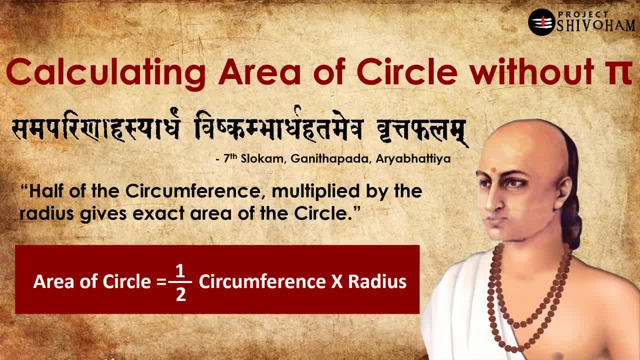 here is just one example from arya bhattia, given by arya bhatta in 500 ce. he gave a formula for calculating the area of a circle without using pi. today, without pi, we can't imagine calculating the area of a circle. it's going to be very, very hectic- not impossible, but very hectic. but back then, like: 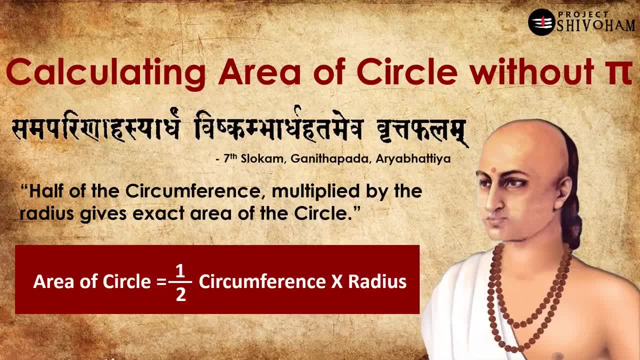 i said, there has been a tradition of measuring things using a rope in india, so with that concept in mind, this formula is easily applicable. what arya bhatta gave. arya bhatta says that the area half of the circumference multiplied by the radius. now, circumference is something that you. 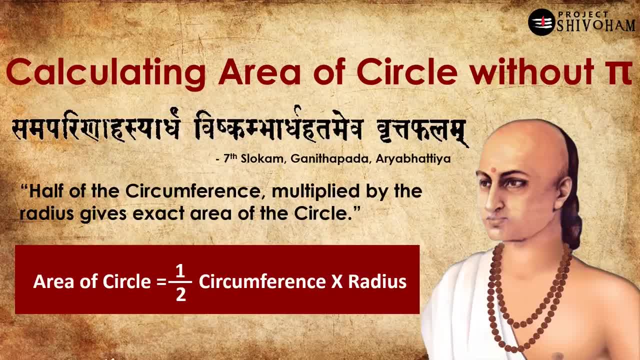 can measure with a row, and the radius as well. so using these the area of a circle can be calculated very easily without touching the value of pi, because pi back then was still in a development mode. you might not get an accurate result if you incorporate pi in your equations and when you're 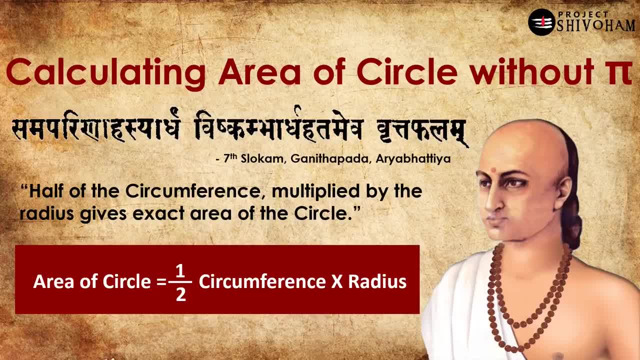 talking about astronomical calculations, even the fourth or fifth place of pi has huge impact. arya bhatta himself gave a better value for pi, but at that time the value given by the chinese was far more accurate than the one which was given by indians. talking about geometry and 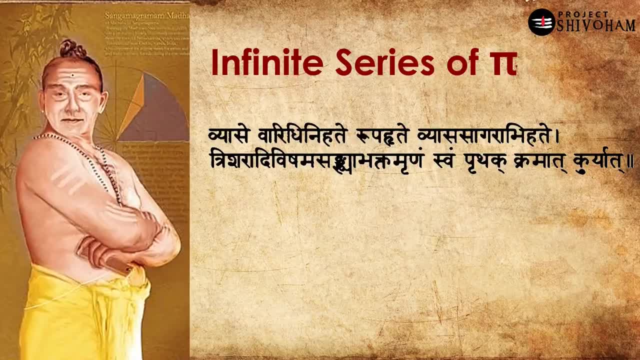 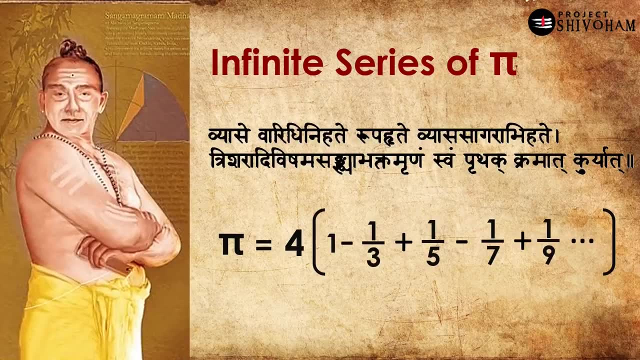 jyotisha together. the most incredible contribution that came from india was in the year 1200, from madhava. people were struggling to find the value of pi, an accurate one, adding up one decimal after other. so the development right from the discovery of the days when greeks first identified that yes, 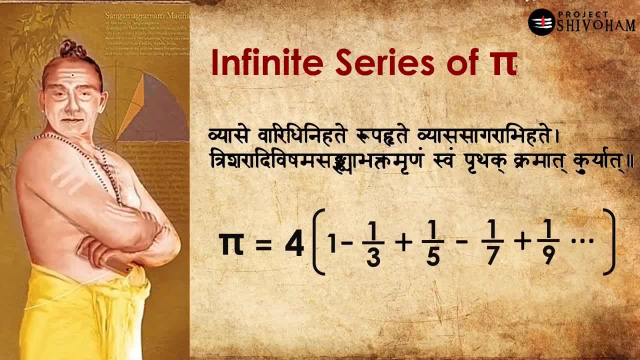 there is a constant like pi, which is a ratio of the circumference to the diameter that can be used in the calculations. the value of pi has been quite irrational, so madhava is the first one to give the value of pi as an infinite series. that means it's up. 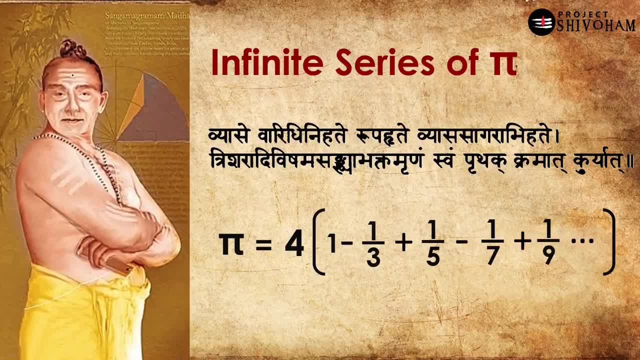 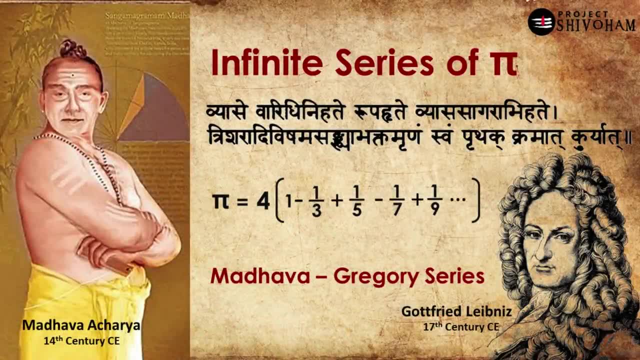 to your patience. you can calculate as much as you want. this is no exaggeration. but this invention is almost as good as landing man on mars. if it's tough for you to believe, read the history of the pi and its evolution and you'll get to know. so madhava gave the value of pi in this small 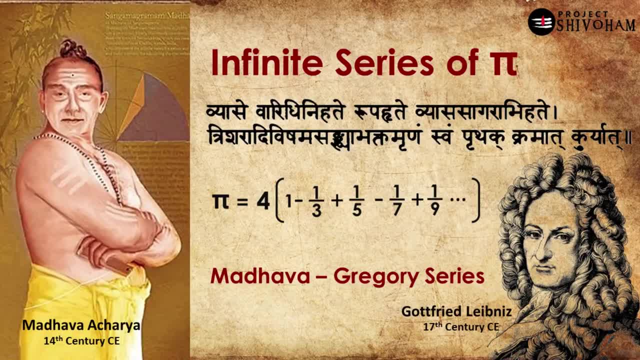 samskritam slocum, so he says that. so, decoding this samskritam slocum, this is what we get: the value of pi. it has now been multiplied by an alternating series of 1 minus 1 by 3 plus 1 by 5 minus 1 by 7. 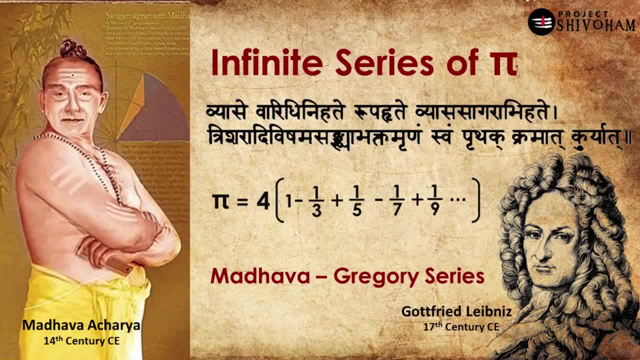 and so on till infinite. in fact, he is the first one to express a finite quantity like pi, in an infinite series. this is one of the fundamental stepping stones of calculus- integration by parts- and this is why i said calculus also has its roots in jyotish, but unfortunately we cannot. 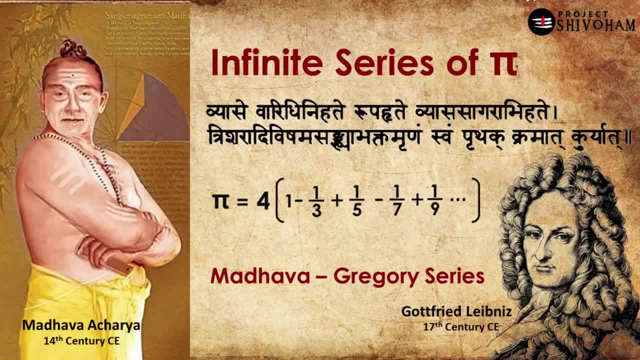 discuss all that now, maybe for some other day. and this series of pi is called as madhava gregory series, which was initially invented by Madhava in the 14th century and reinvented by Gottfried Leibniz in 17th century, So in his 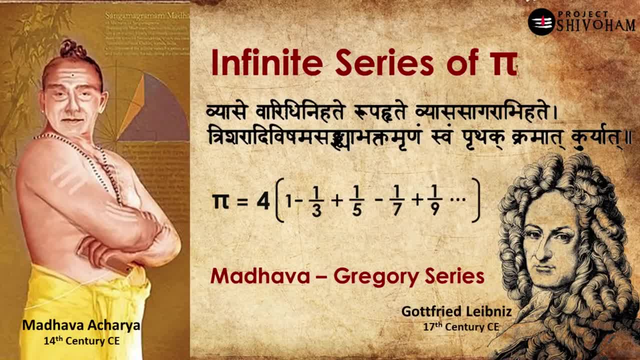 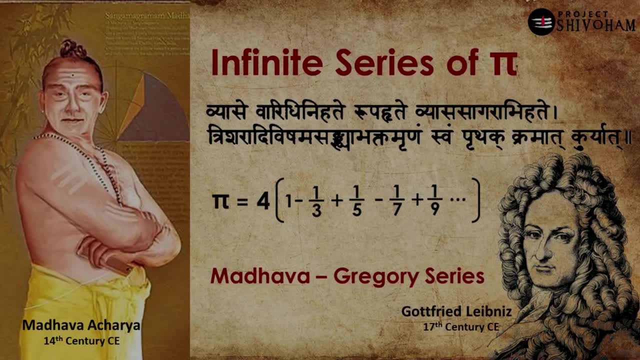 honor, the series is named after Madhava, as well as Gregory. saying that Madhava-Gregory series. Again, a vast majority of us are not aware of this, for obvious reasons. Up next is geometry in Shilpa Shastra. 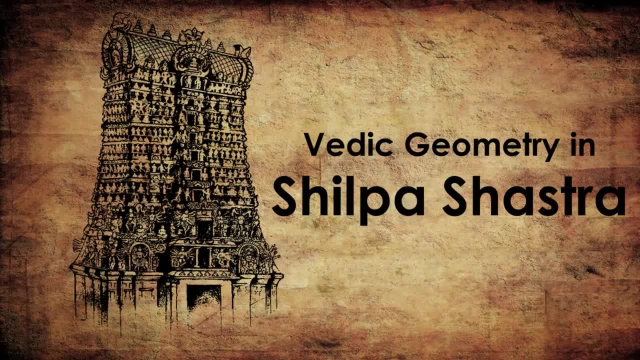 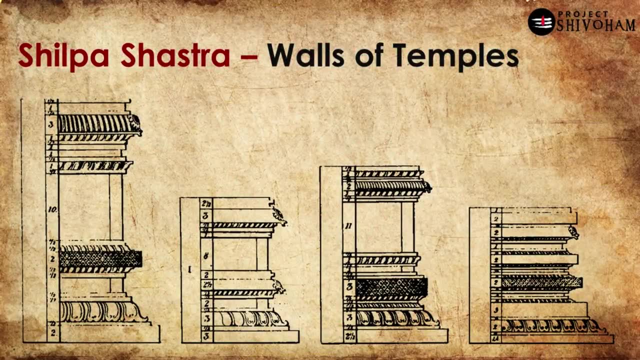 Temples, the epicenter of Indian art, culture and heritage. So beautiful are the carvings and the sculptures, but what's actually behind them? Let's quickly have a look. Unlike Jyotish Shastra and Kalpa, the geometrical concepts of Shilpa Shastra is not really something. 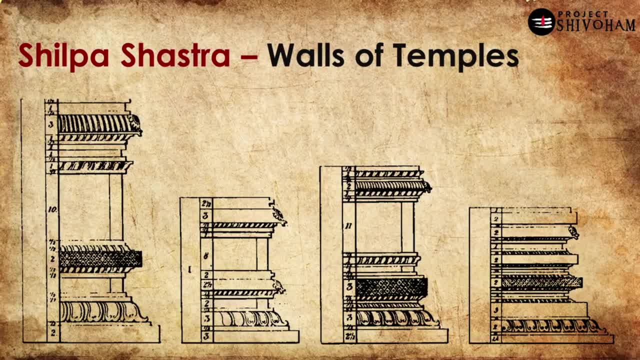 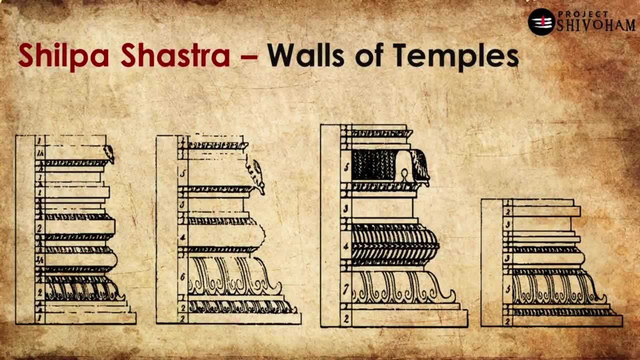 that we could possibly use or try to understand. It is so intricate and blended with the way the sculptings are done. So here you see, as an example, the walls of a temple. There are different varieties of designs depending on the deity of the temple. There are specified designs. 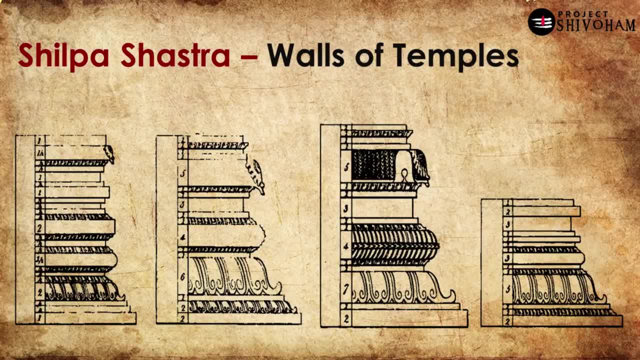 not just any random ones, to be carved in accordance with the scriptures of Agama, Manasara or Sita. These are different books which describe how a temple construction needs to be done. Shilpa Shastra also gives the geometrical guidelines about constructing and carving. 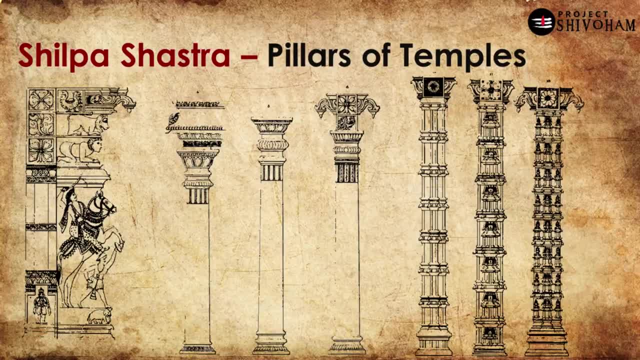 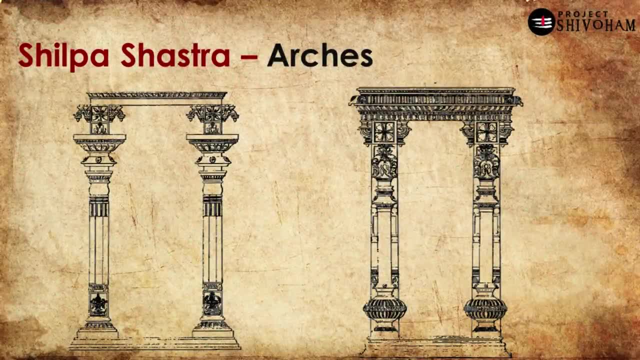 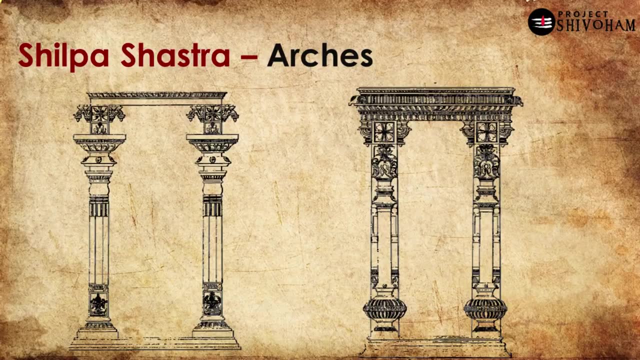 different kinds of pillars. as you see here, It gives the structural guidelines as well as the aesthetic guidelines in building the pillars and other parts of the temple, And here are some blueprints about the arches that would be constructed in the temple. The interesting part is all these designs are explained in form of Samskritam slokams. It's 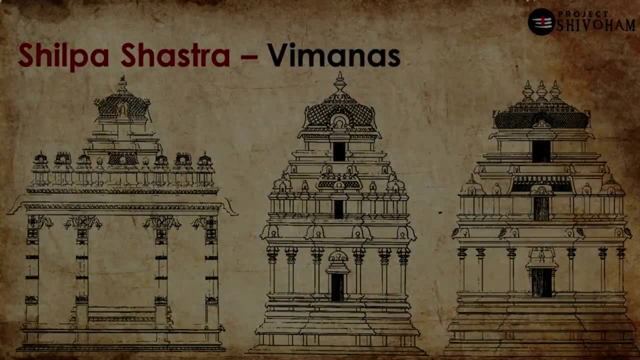 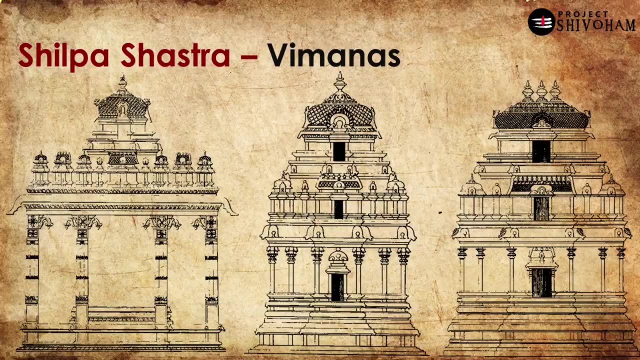 quite interesting to see how they are constructed. Shilpa Shastra also explains how such great details are encoded in Samskritam. Here are the most catchy parts of the temple: the Vimanas or the Gopuram. Shilpa Shastra explains great detail about how these need to be layered and sculpted. 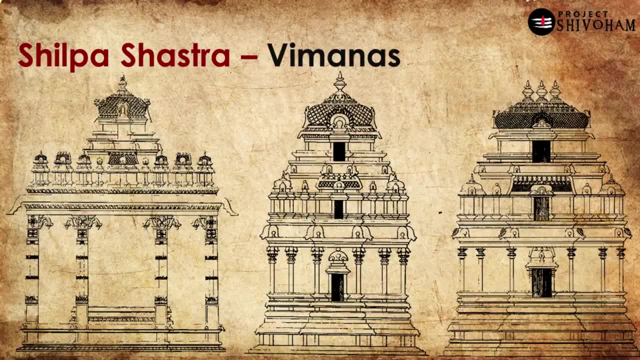 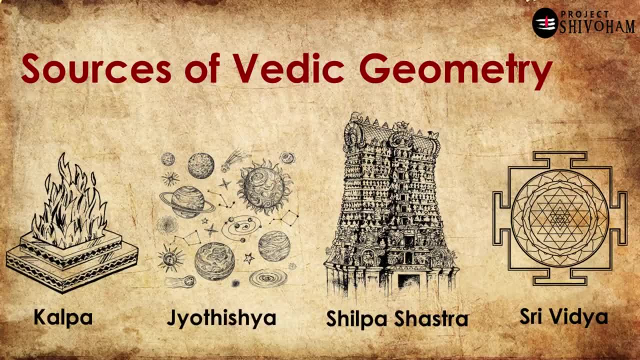 both for its structure as well as for its aesthetics, And in all, geometrical principles are well blended in each of them. There we have the last category, Srividya, which also has complex geometrical procedures blended into it. Srividya is a path of devotion in which Srividya 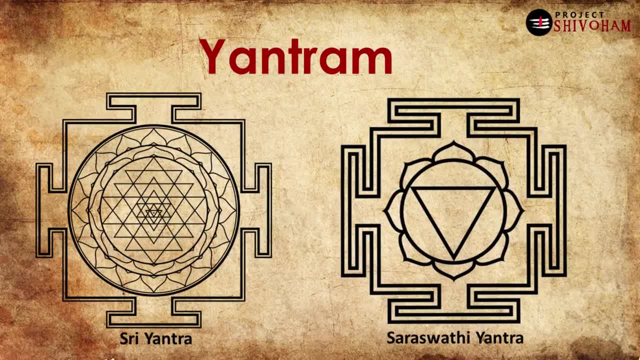 Lalita Parameshwari is worshipped as the epitome of the nature and the cosmos. As part of this practice, what you're seeing on the screen are called as yantras. These yantras are manifestation of the gods themselves. So that's what the practice is all about: People. 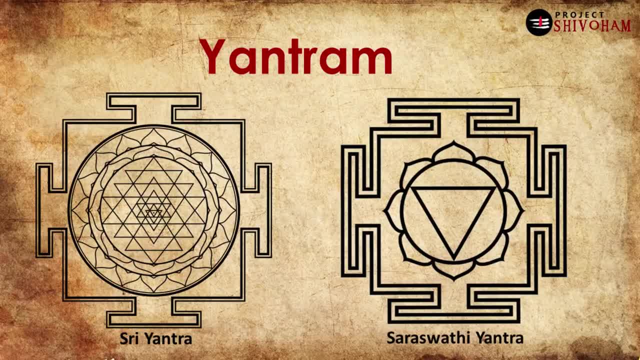 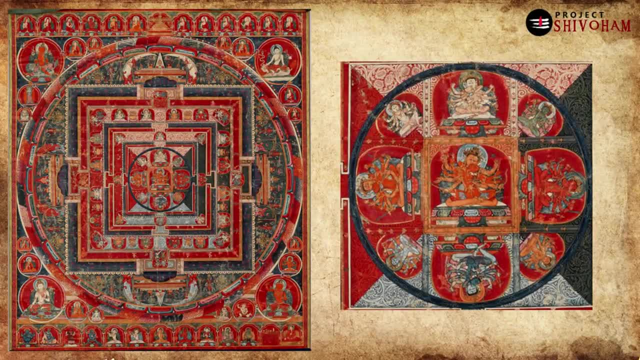 meditate on these yantras as part of their spiritual process. But as we are looking from a geometry standpoint, we'll see it from that angle To understand these geometrical diagrams called yantras. basically, they are revered as a layout. in each vertex line corner holds a deity, And it's like a labyrinth where people start meditating. 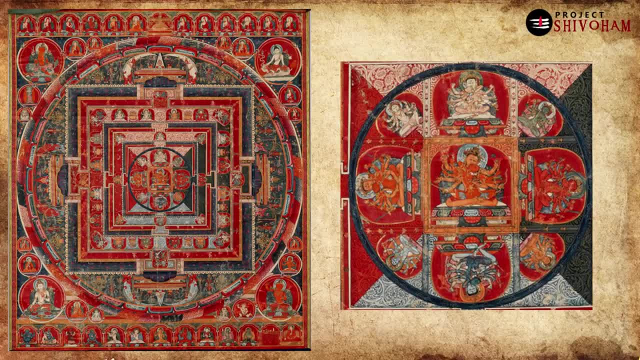 through their paths, navigating towards the center of the yantra. It's a bit complicated and I myself don't have a clear-cut understanding about the spiritual aspects of it, So let's limit ourselves from the geometry standpoint. The most important topic here is, as you see, 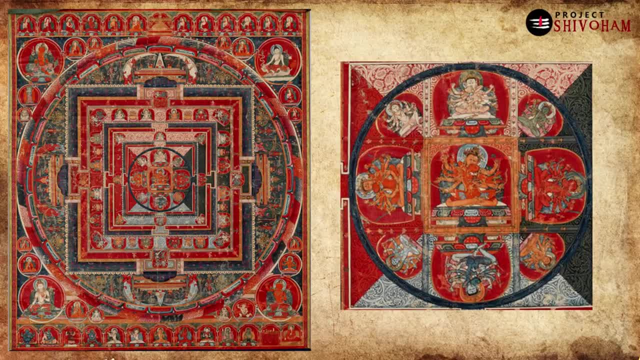 we have a lot of deities in each and every space of this diagram, So that translates to incredible precision in the geometrical structures which are the yantras. So to create these geometrical structures, or the yantras, a lot of techniques have originated in building these. 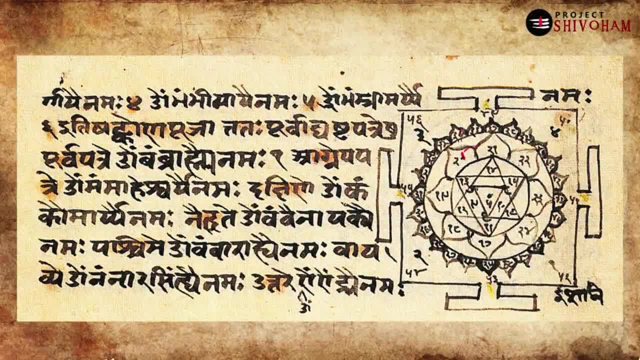 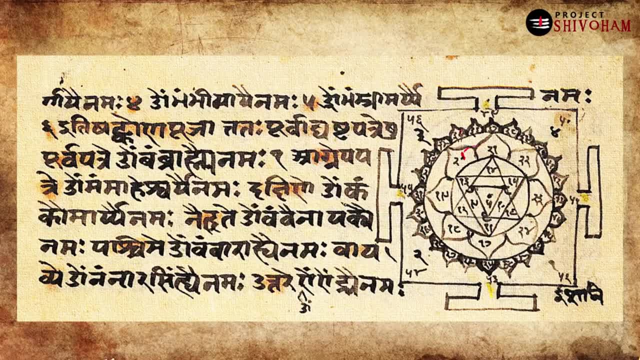 diagrams. And this is a very, very ancient culture And there are many temples where you have these yantras carved into either the floor or the ceiling or in other parts of the temples. Here is a manuscript detailing out some yantra and describing the way one has to follow it. It's just a snippet. 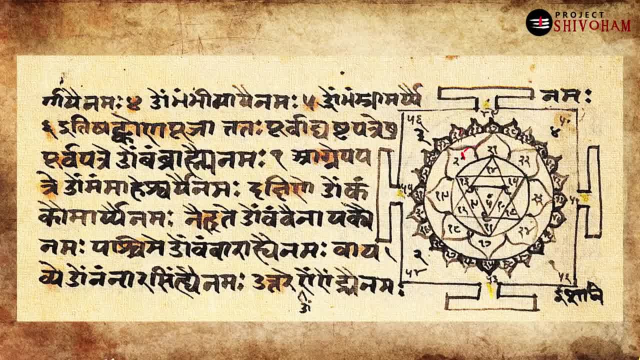 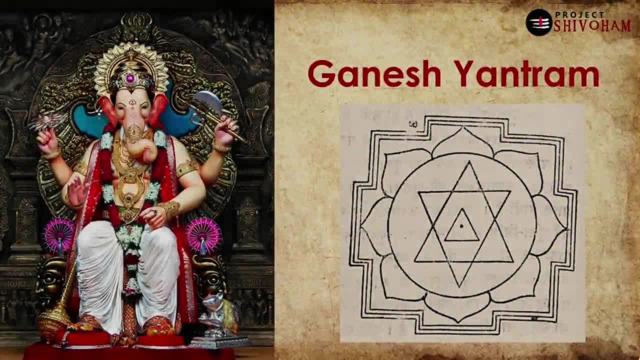 from a very ancient manuscript. You see here the diagrams, how they are drawn. These diagrams show the way one chooses to worship in his or her path of devotion. So here is a specific example of Ganesha yantra, which is a manifestation of Lord Ganesha himself. So that's what and how it. 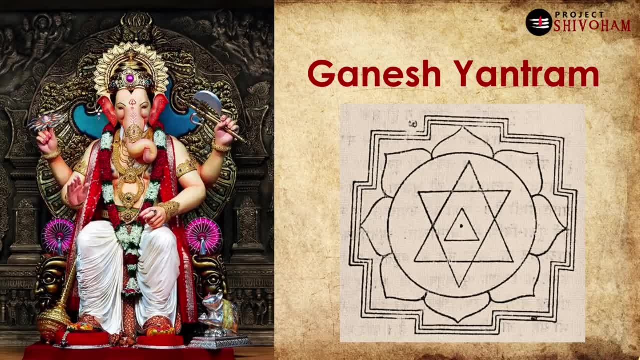 is revered, And this is just a rough sketch, but when it comes to actually consecrating such kind of a yantra, a high geometric precession is ensured And as part of it, there are a lot of construction techniques as part of the Vedic geometry that designs these yantras And this one. 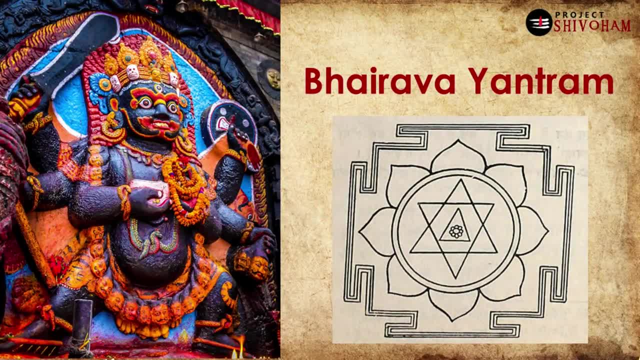 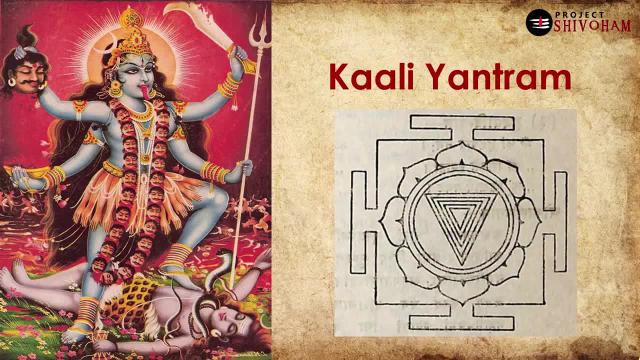 is a Bhairava yantra manifestation of Lord Shiva in the form of Bhairava, one of Bhairava's yantras, The most ferocious forms of Lord Shiva, And this yantra is Mahakali yantra, which is a manifestation. 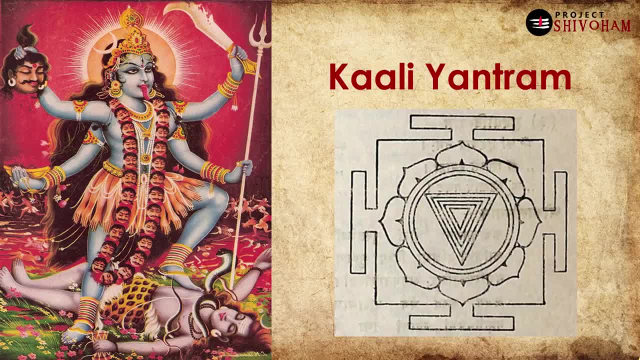 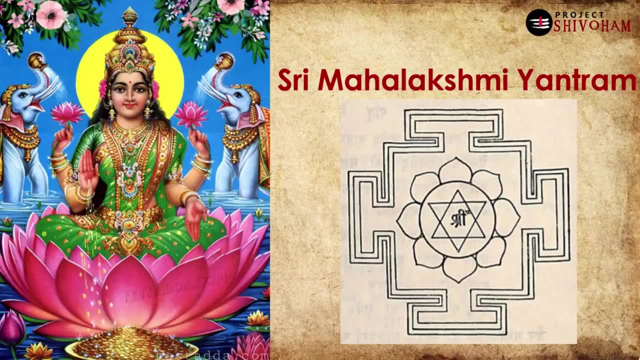 of Kalima. These look like simple diagrams, but the proportions and precession and the symmetricity, they matter a lot when it comes to consecrating them. This one is Sri Mahalakshmi yantra, again a manifestation of Goddess, Sri Mahalakshmi, And of all the yantras, Sri yantra. 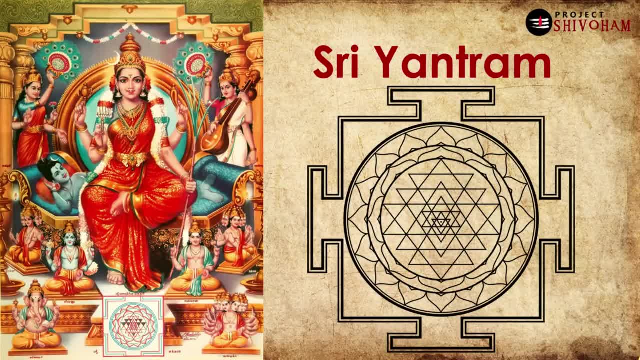 is revered as the most important yantra when it comes to Srividya, And it's a highly complex structure where the precession matters to the pixel. It has nine triangles, which shows as a confluence of Shiva and Shakti holding the topmost importance in the spiritual process. There is a lot. 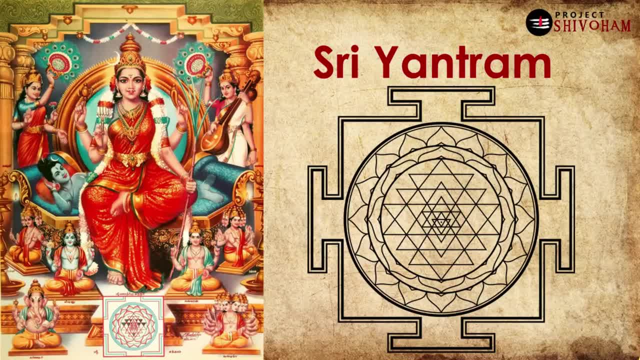 of mathematical analysis that was done in many universities across India, Europe and US on Sri Chakra and its symmetricity and other geometrical properties. At this point in time I don't fully understand it, And the day I understand we'll definitely do a detailed documentary about it. 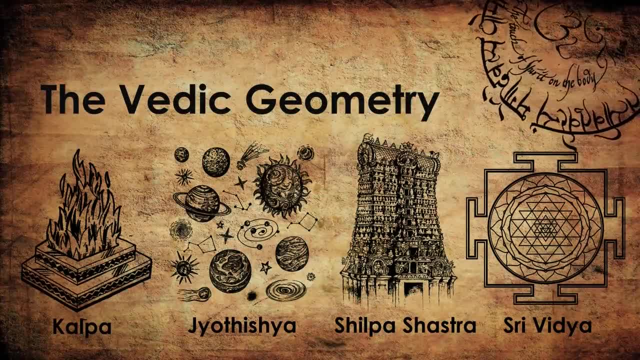 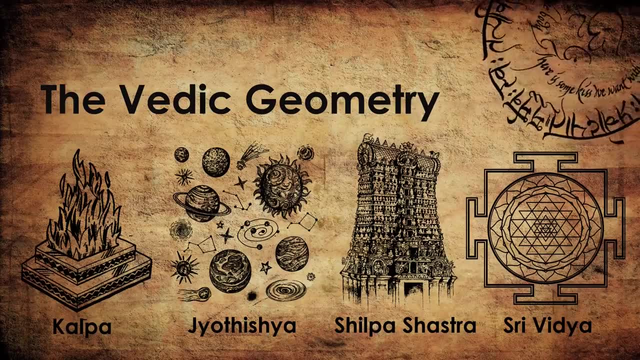 Well, now, that's a very brief overview about Sri Mahalakshmi yantra and how it pans across all these four areas. I'd like to come back to Sulbha Sutras again. I was really surprised to learn the fact that it is the world's oldest.